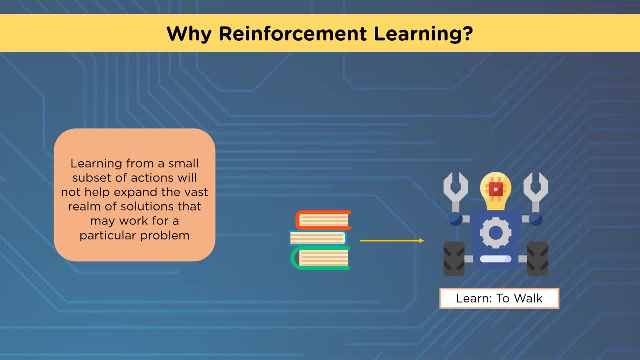 of actions will not help expand the vast realm of solutions that may work for a particular problem. You can see, here we have the robot learning to walk- Very complicated setup. when you're learning how to walk, You'll start asking questions like if I'm taking one step. 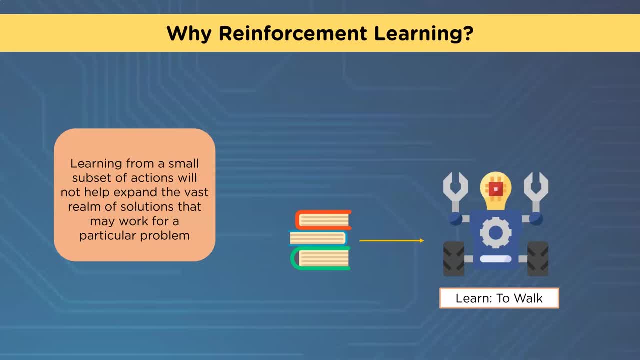 forward and left. what happens if I pick up a 50-pound object? How does that change how a robot would walk? And these things are very difficult to program because there's no actual information on it until it's actually tried out. Learning from a small subset of actions will not help expand. 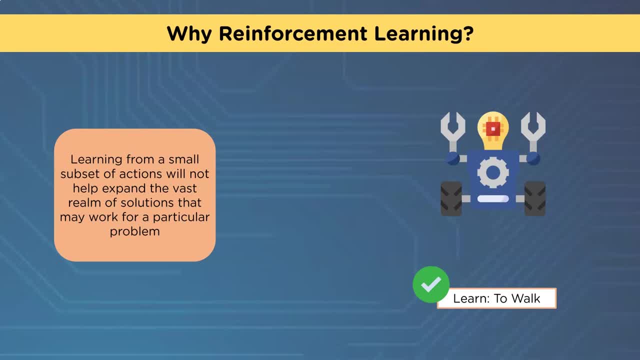 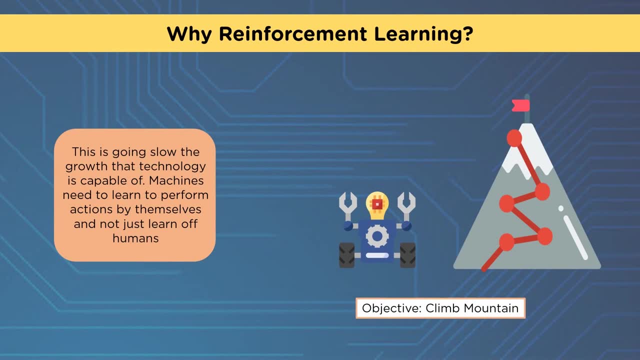 the vast realm of solutions that may work for a particular problem, And we'll see here. it learned how to walk. This is going to slow the growth that technology is capable of. Machines need to learn to perform actions by themselves and not just learn off humans. 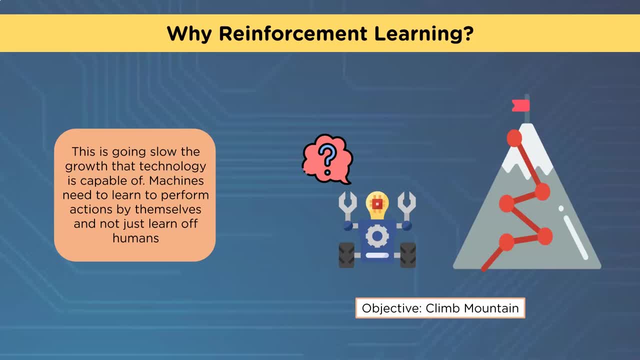 And you see the objective: climb a mountain. The real interesting point here is that as human beings we can go into a very unknown environment and we can adjust for it and kind of explore and play with it. Most of the models, the non-reinforcement models in computer machine learning, aren't able to do that very. 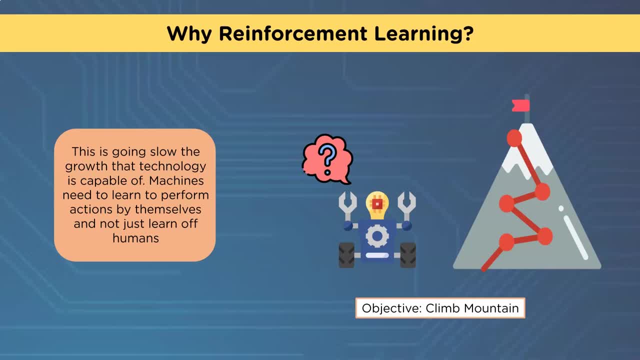 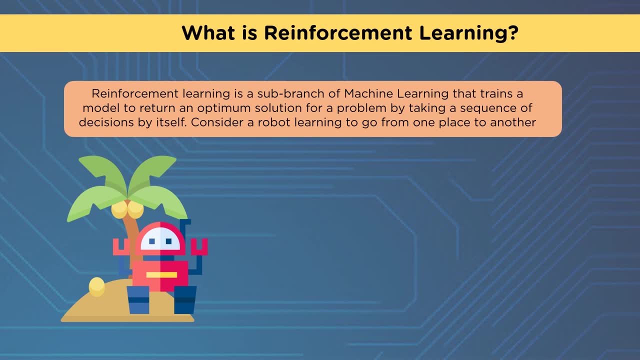 well, There's a couple of them that can be used or integrated. See how it goes is what we're talking about with reinforcement learning. So what is reinforcement learning? Reinforcement learning is a sub-branch of machine learning that trains the model to 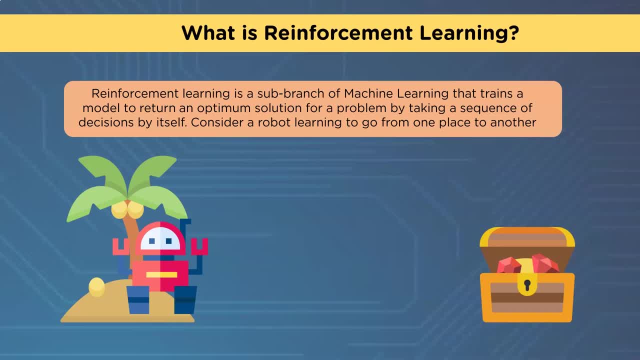 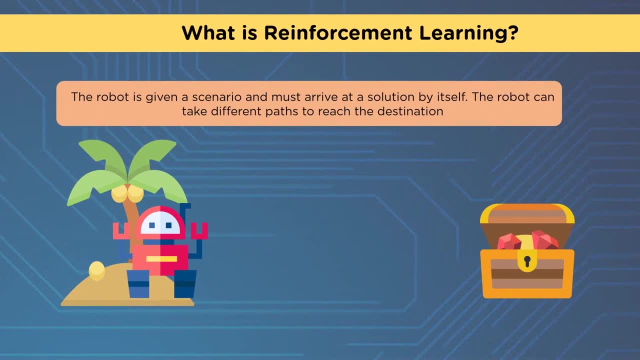 return an optimum solution for a problem by taking a sequence of decisions by itself. Consider a robot learning to go from one place to another. The robot is given a scenario and must arrive at a solution by itself. The robot can take different paths to reach the. 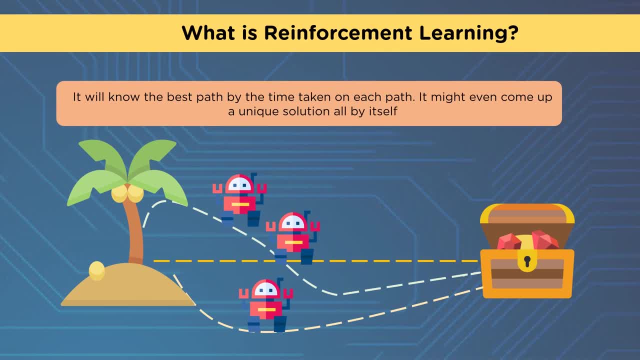 destination. It will know the best path by the time taken on each path and might even come up with a unique solution all by itself, And that's really important, as we're looking for unique solutions. We want the best solution, but you can't find it unless you try it. 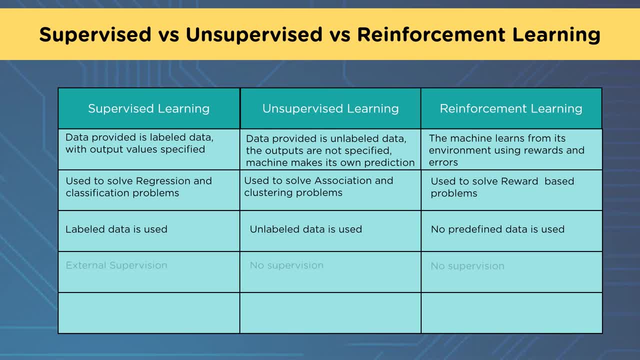 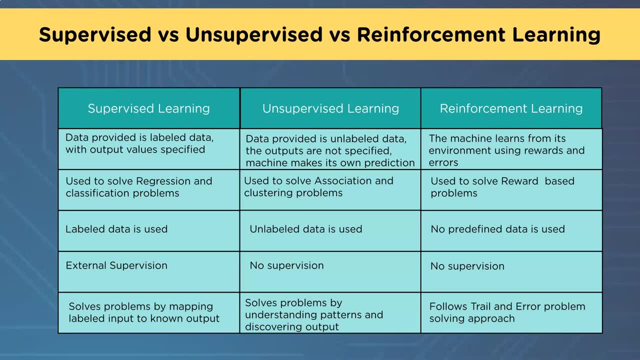 So we're looking at our different systems, our different model. We have supervised versus unsupervised, versus reinforcement learning, And with the supervised learning that is probably the most controlled environment. We have a lot of different supervised learning models, whether it's linear, regression, neural. 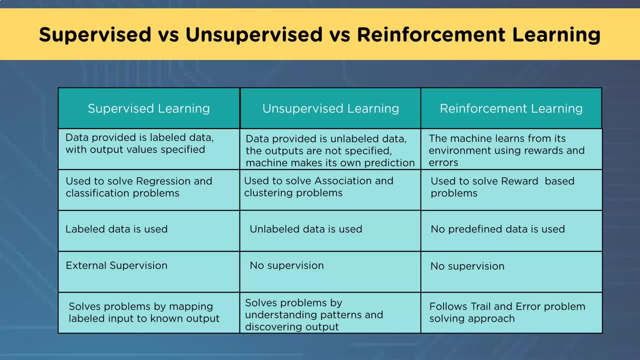 networks. there's all kinds of things in between decision trees. The data provided in the model is labeled data with output values specified, And this is important because when we talk about supervised learning, you already know the answer for all this information. You already know the picture has a motorcycle in it, So 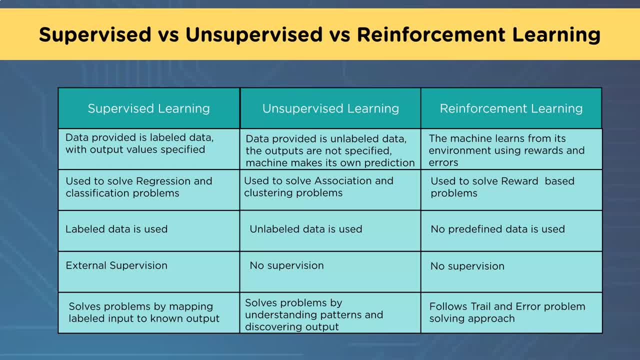 you're supervised, learning. You already know that the outcome for tomorrow, for going back a week, you're looking at stock. you can already have like the graph of what the next day looks like, So you have an answer for it And you have labeled data which is used. You have an external supervision and solves problems. 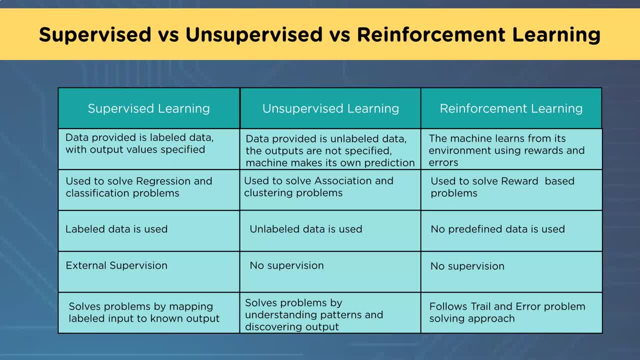 by mapping labeled input to known output. So very controlled Unsupervised learning. and unsupervised learning is really interesting because it's now taking part in many other models. They start with an. you can actually insert an unsupervised learning model in almost either supervised or reinforcement learning as part of the system. 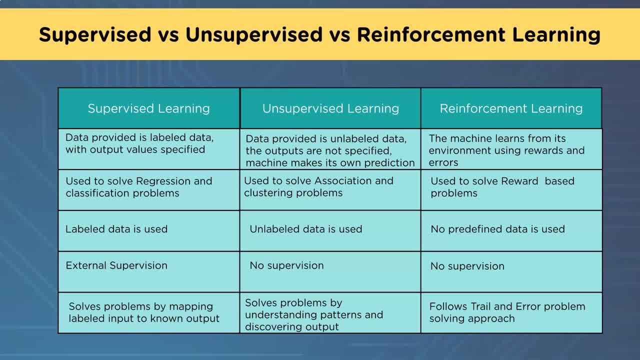 which is really cool. Data provided is unlabeled data. The outputs are not specified. Machine makes its own predictions. Used to solve association with clustering problems. Unlabeled data is used. No supervision Solves problems by understanding patterns and discovering output. 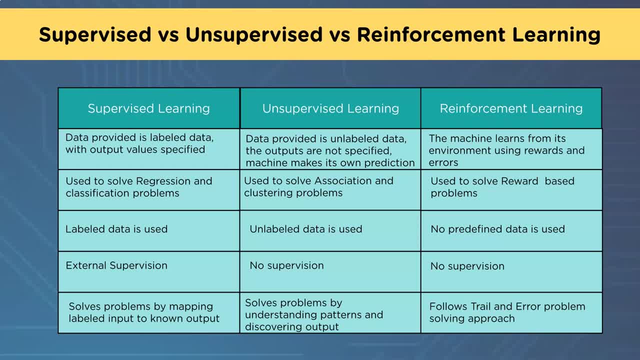 So you can look at this and you can think some of these things go with each other. They belong together. So it's looking for what connects in different ways And there's a lot of different algorithms that look at this. When you start getting into those, there's some really cool images that come up of what 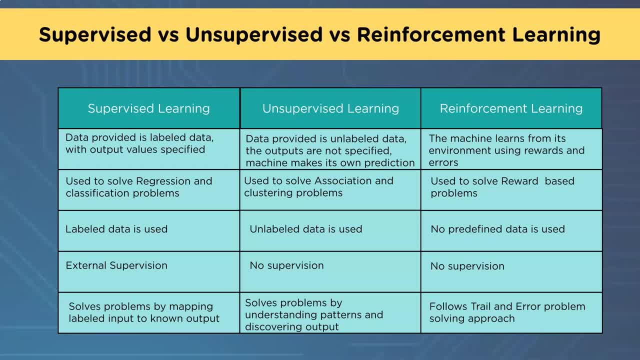 unsupervised learning is How it can pick out, say, the area of a donut. One model will see the area of the donut and the other one will divide it into three sections based on its location versus what's next to it. 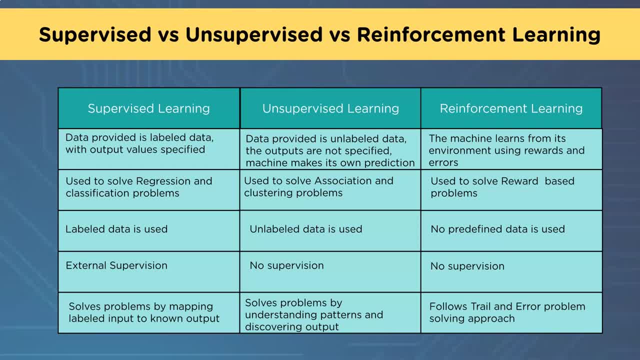 So there's a lot of stuff that goes in with unsupervised learning, And then we're looking at reinforcement learning, Probably the biggest industry in today's market in machine learning or growing market. it's very infant stage as far as how it works and 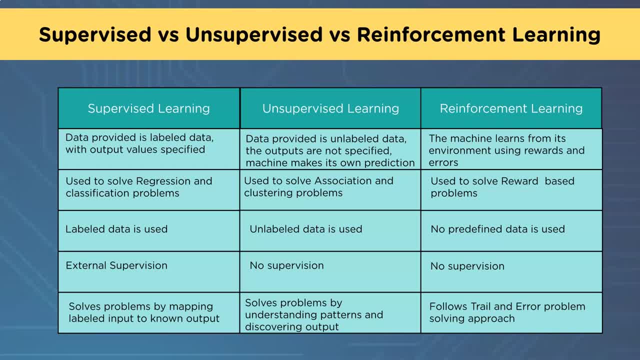 what it's going to be capable of. The machine learns from its environment using rewards, Rewards and errors used to solve reward-based problems. No predefined data is used, No supervision Follows trail and error problem solving approach. So again we have a random. At first, you start with a random. I try this, It works, and this: 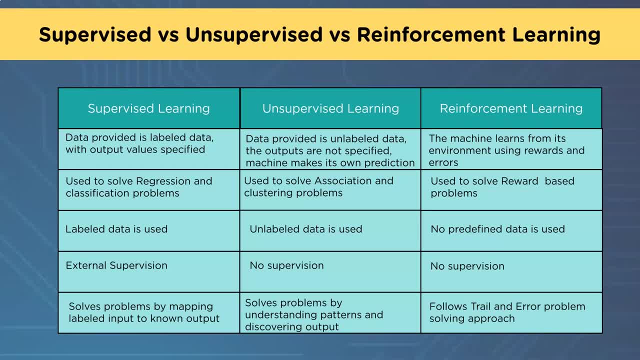 is, my reward Doesn't work very well. maybe, Or maybe it doesn't even get you where you're trying to get it to do And you get your reward back. And then it looks at that and says: well, let's try something. 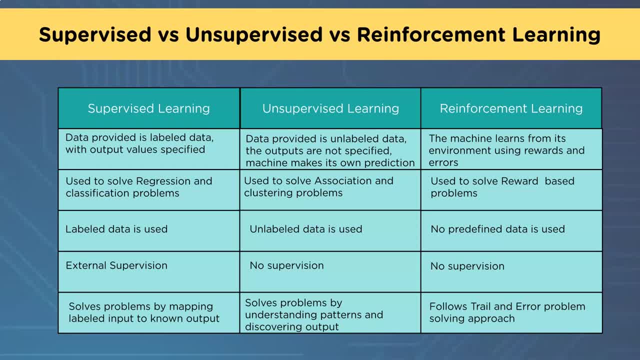 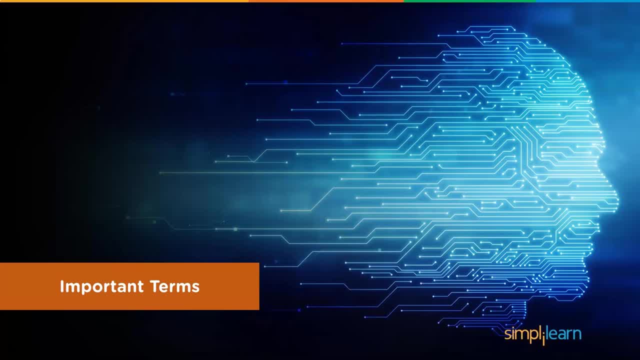 else And it starts to play with these different things finding the best route. So let's take a look at important terms in today's reinforcement model, And this has become pretty standardized over the last few years, So these are really good to know. 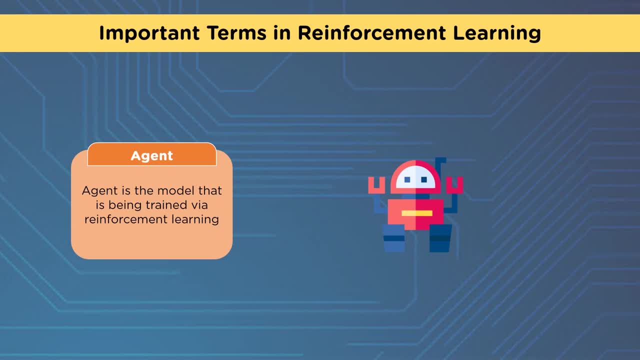 We have the agent. Agent is the model that is being trained via reinforcement learning. So this is your actual entity that has, however you're doing it, whether you're using a neural network or a cue table or whatever combination thereof, this is the actual agent that you're. 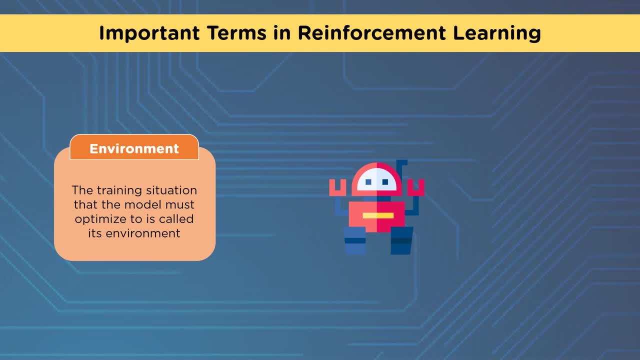 using. This is the model, And you have your environment. The training situation that the model must optimize to is called its environment, And you can see here: I guess we have a robot who's trying to get a chest full of gems or whatever, and that's the output. 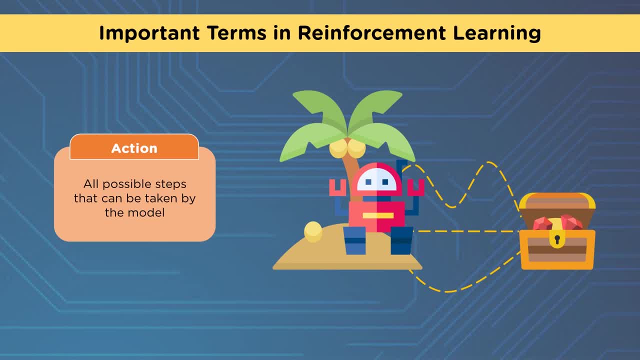 And then you have your action. This is all possible steps that can be taken by the model And it picks one action And you can see here that it's picked three different routes to get to the chest of diamonds and gems. We have a state, the current position, condition returned by the model. 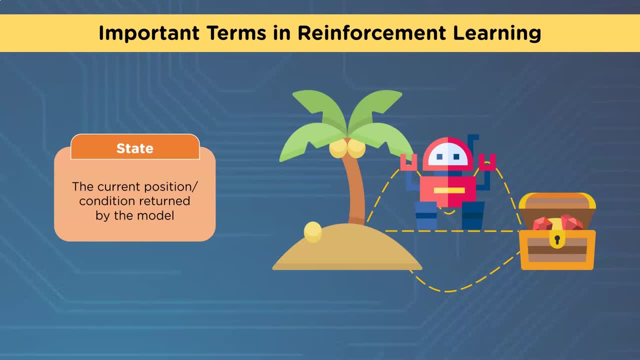 And you can look at this. if you're playing like a video game, this is the screen you're looking at. So when you go back here, the environment is a whole game board. So if you're playing one of those Mobius games, you might have the whole game board. 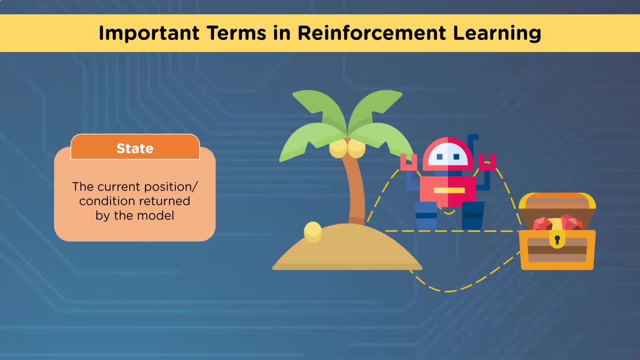 going on, but then you have your current position. Where are you on that game board? What's around that? What's around you? If you were talking about a robot, the environment might be moving around the yard. where it is in the yard. 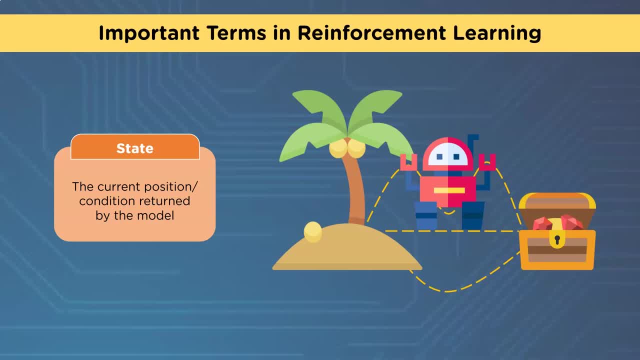 And you can see what input it has in that location. That would be the current position condition returned by the model. And then the reward: To help the model move in the right direction, it is rewarded, Points are given to it to appraise some kind of action. 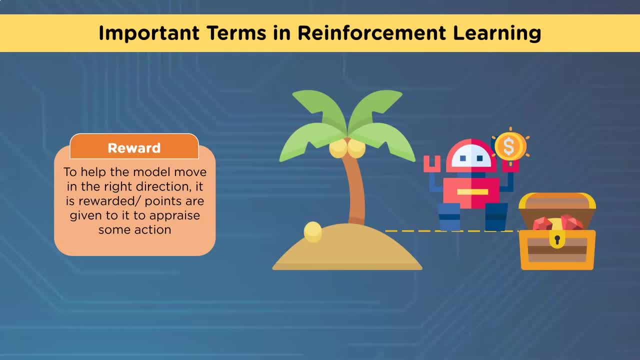 So yeah, you did good, Or if it didn't do as good, trying to maximize the reward and have the best reward possible. And then policy. Policy determines how an agent will behave at any time. It acts as a mapping between action. 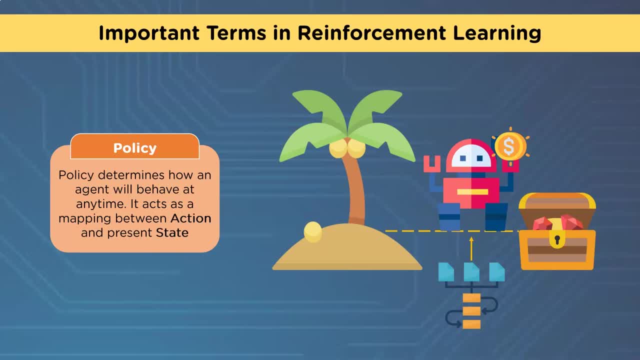 This is part of the model. What is your action that you're going to take? What's the policy you're using to have an output from your agent? One of the reasons they separate policy as its own entity is that you usually have a prediction of different options. 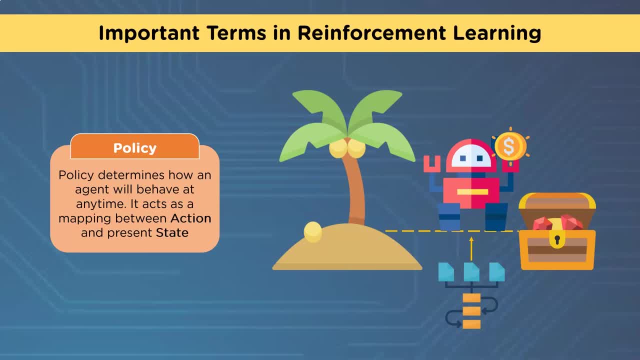 And then the policy. well, how am I going to pick the best Based on those predictions? I'm going to guess at different options and we'll actually weigh those options in And find the best option we think will work. So it's a little tricky, but the policy thing is actually pretty cool how it works. 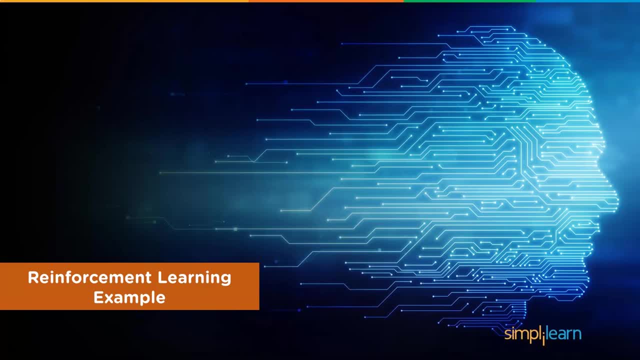 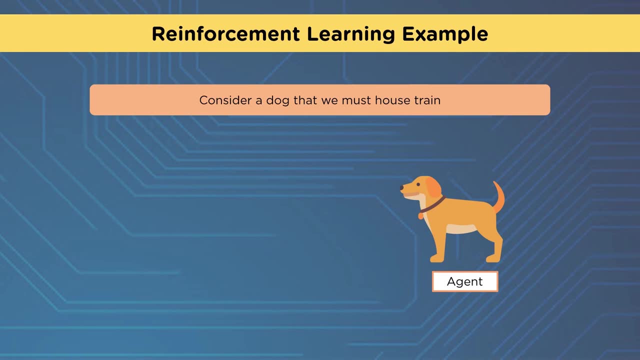 Let's go ahead and take a look at a reinforcement learning example And just in looking at this we're going to take a look, consider what a dog that we want to train. So the dog would be like the agent. So you have your puppy or whatever. 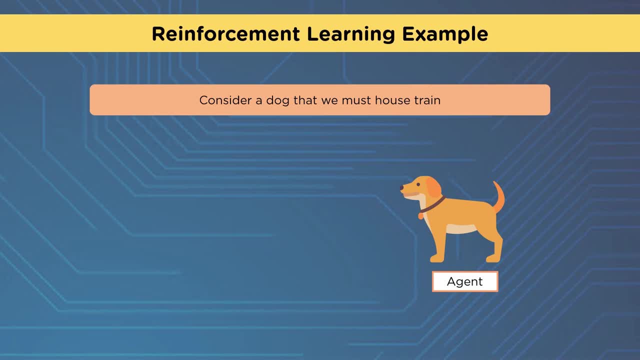 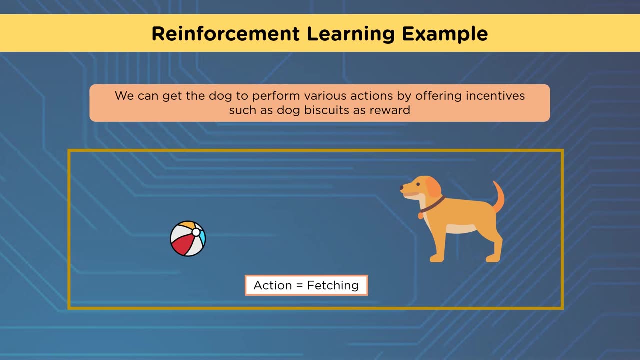 And then your environment is going to be the whole house or whatever it is where you're training them. And then you have an action: We want to teach the dog, We want the dog to fetch. So action equals fetching. And then we have a little biscuit. 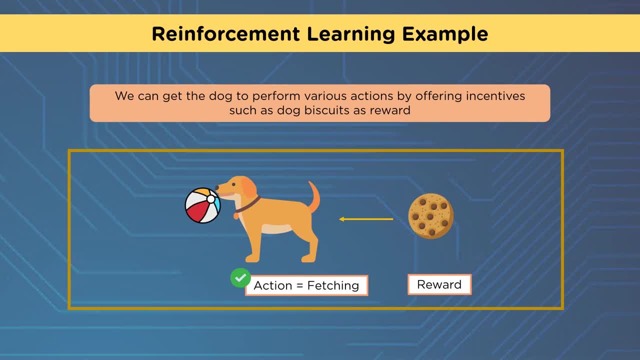 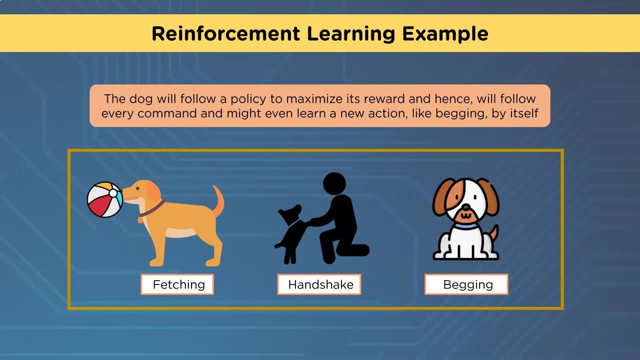 So we can get the dog to perform various actions by offering incentives, such as a dog biscuit as a reward. The dog will follow a policy to maximize this reward and hence will follow every command and might even learn new actions, like begging, by itself. So we started off with fetching. 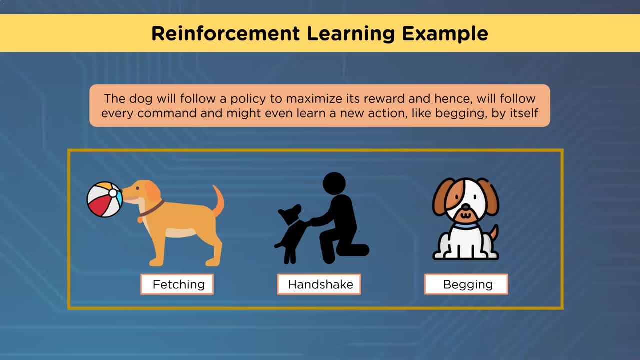 It goes: oh, I get a biscuit for that. It tries something else And you get a handshake or begging or something like that, And it goes: oh, this is also reward-based, And so it kind of explores things to find out what will bring it its biscuit. 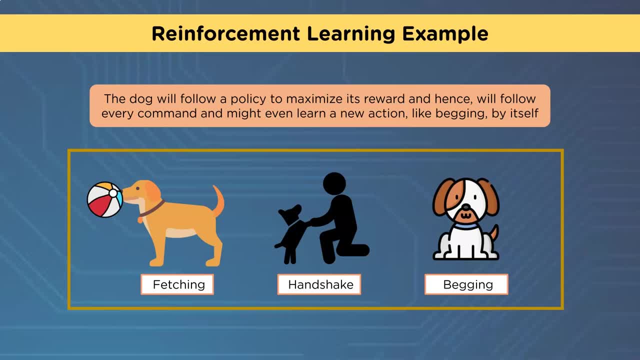 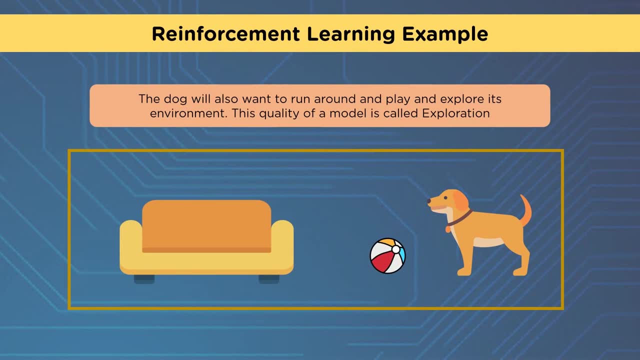 And that's very much like how a reinforced model goes- is it looks for different rewards. How do I find, can I try different things and find a reward that works? The dog also will want to run around and play in an explorer's environment. 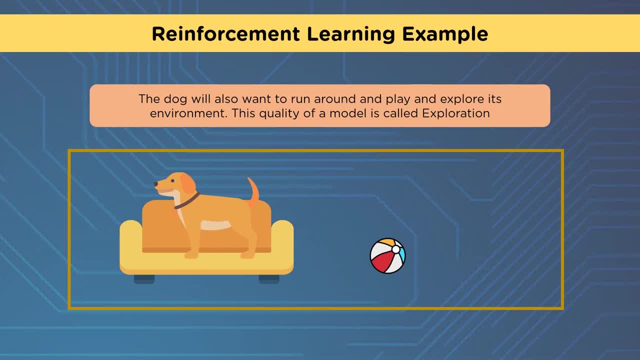 This quality of model is called exploration. So there's a little randomness going on in exploration And it explores new parts of the environment. It's going to explore new things. It's going to explore new things. It's going to explore new parts of the house. 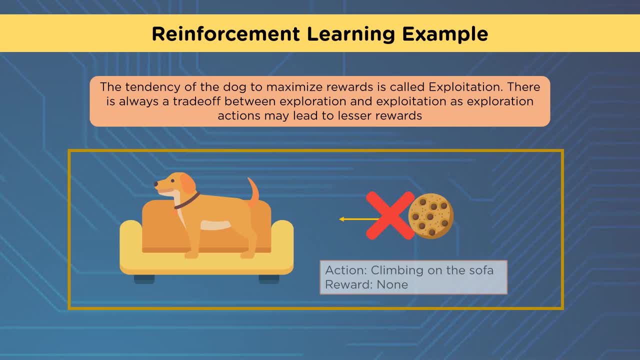 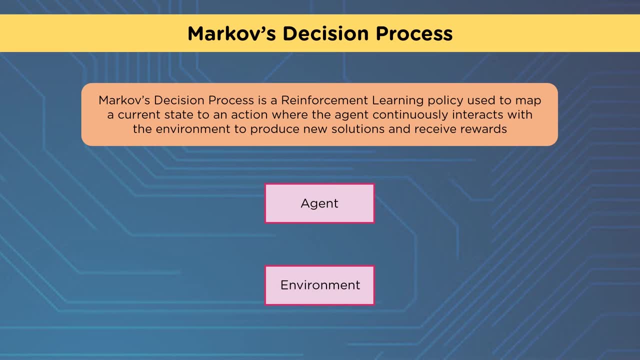 Climbing on the sofa doesn't get a reward. In fact, it usually gets kicked off the sofa. So let's talk a little bit about Markov's Decision Process. Markov's Decision Process is a reinforcement learning policy used to map a current state. 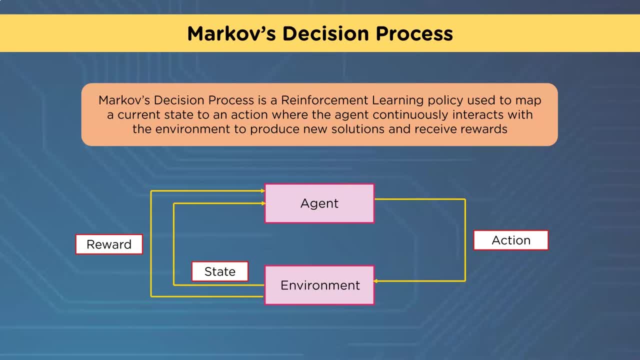 to an action where the agent continuously interacts with the environment to produce new solutions and receive rewards. And you'll see- here's all of our different vocabulary we just went over. We have a reward state or agent or environment interaction, And so even though the environment kind of contains- 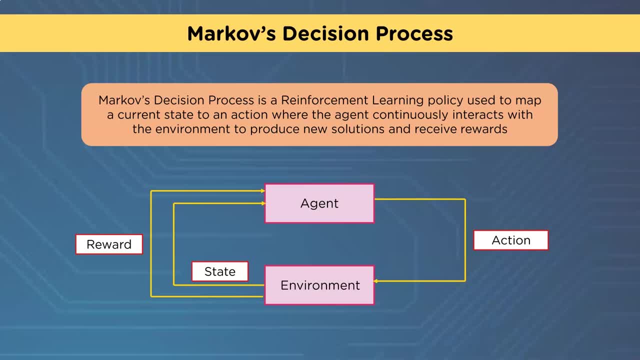 everything that you really, when you're actually writing the program, your environment's going to put out a reward in state that goes into the agent. The agent then looks at this state or looks at the reward, usually first and it says, okay, I got rewarded for whatever I just did. 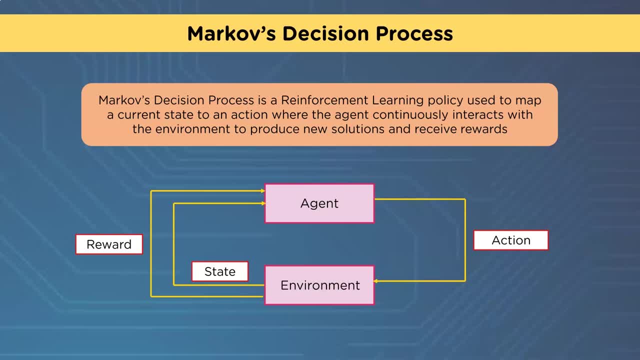 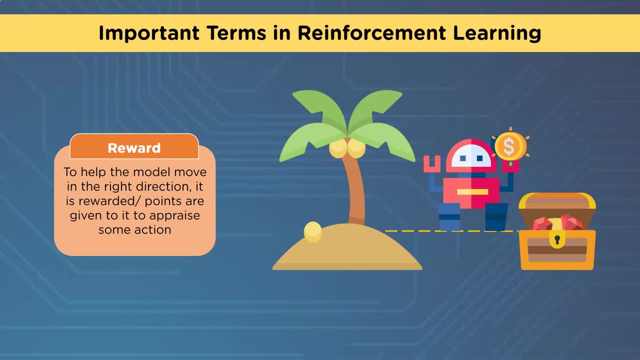 or it didn't get rewarded. And then it looks at the state and then it comes back And if you remember from policy, the policy comes in and then we have a reward. The policy is that part that's connected at the bottom. And so it looks at that policy and it says, hey, what's a good. 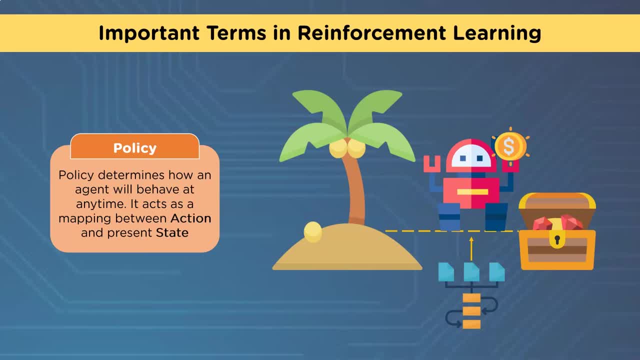 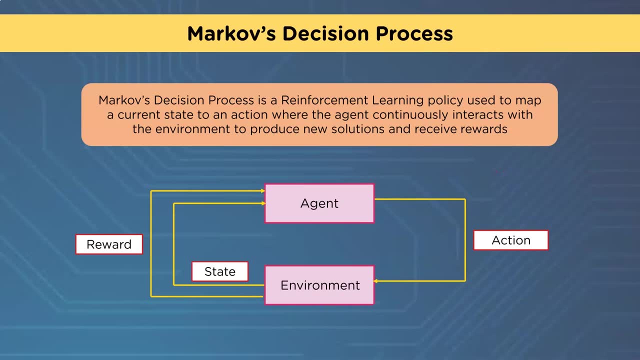 action that will probably be similar to what I did, or sometimes they're completely random, but what's a good action that's going to bring me a different reward. So taking the time to just understand these different pieces as they go is pretty important in most of the models today. 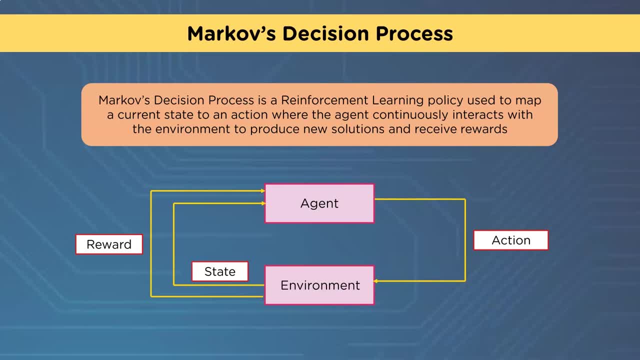 And so a lot of them actually have templates based on this that you can pull in and start using- Pretty straightforward as far as once you start seeing how it works, you can see your environment sends. it says: hey, this is what the agent did this. If you're a character in a game, this happened. 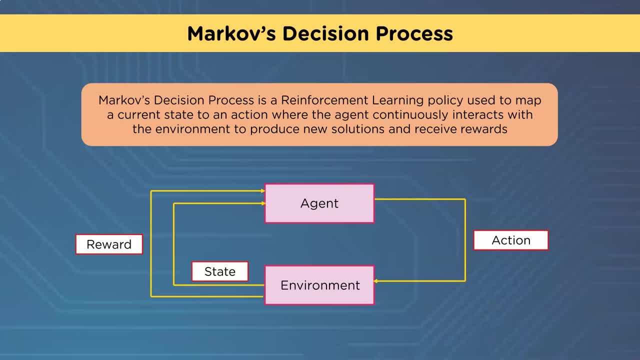 and it shoots out a reward in a state. The agent looks at the reward, looks at the new state and then takes a little guess and says: I'm going to try this action. And then that action goes back into the environment. It affects the environment. The environment then changes depending on what the 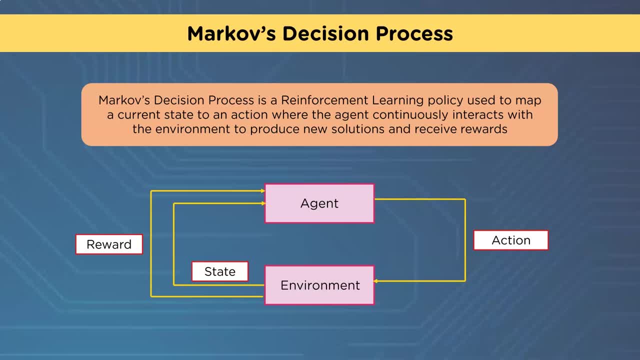 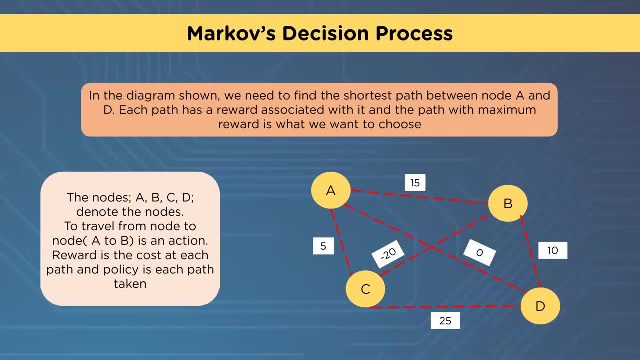 action was, And then it has a new state and a new reward that goes back to the agent. So in the diagram shown we need to find the shortest path between node A and D. Each path has a reward associated with it and the path with a maximum reward is what we want to choose: The nodes A, B, C. 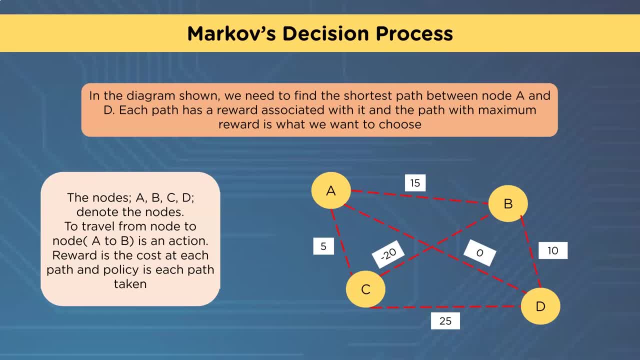 D denote the nodes. to travel from node A to B is an action. Reward is the cost of each path and policy is each path taken. And you can see here: a could go to B or a can go to C right off the bat or it can go right to D. And if you explored all three of these you would find 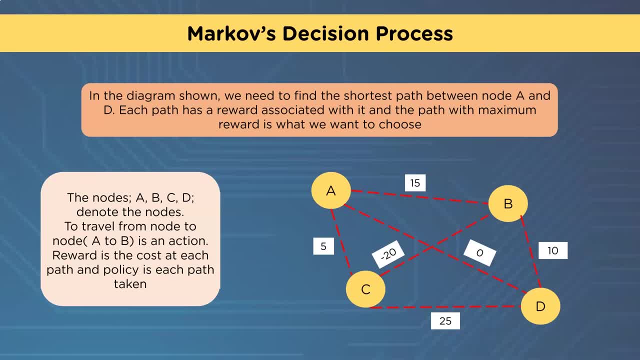 that A going to D was a zero reward. 0, 3, C and D would generate a different reward, or you could go A, C, B, D. There's a lot of options here, And so when we start looking at this diagram, you start to realize that 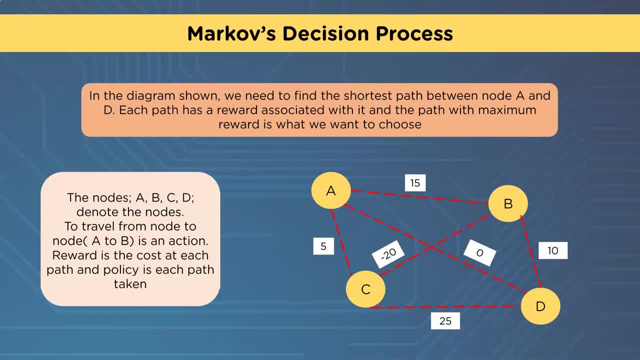 even though today's reinforced learning models do really good at finding an answer, they end up trying almost all the different directions, you see, And so they take up a lot of work or a lot of processing time for reinforcement learning. They're right now in their infant. 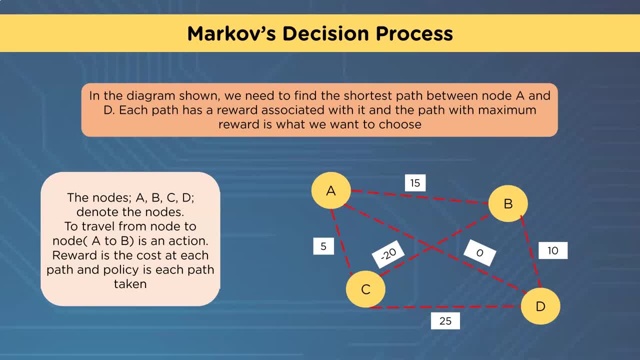 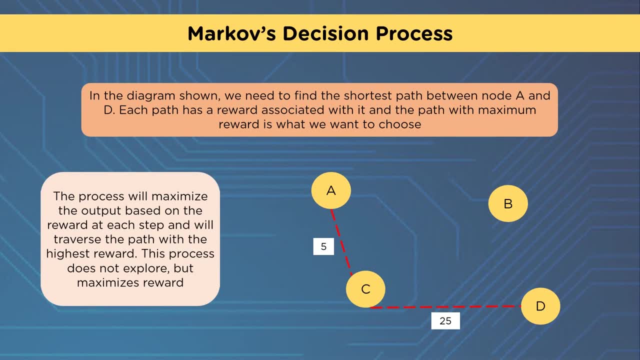 stage and they're really good at solving simple problems And we'll take a look at one of those in just a minute in a tic-tac-toe game. But you can see here, once it's gone through these and it's explored it's going to find the A, C, D is the best reward It. 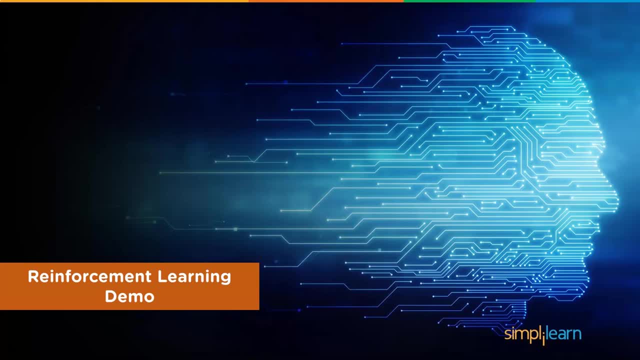 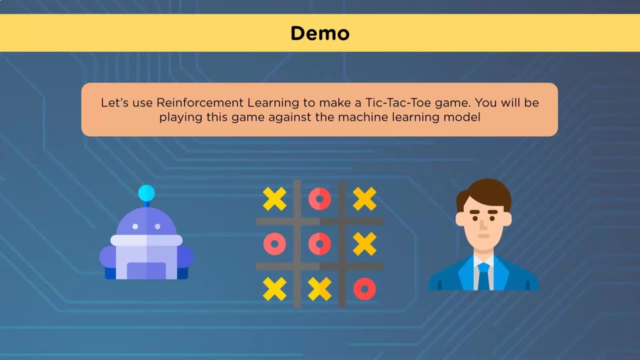 gets a full 30 points for it. So let's go ahead and take a look at a reinforcement learning demo. In this demo, we're going to use reinforcement learning to make a tic-tac-toe game. You'll be playing this game against the machine learning model. 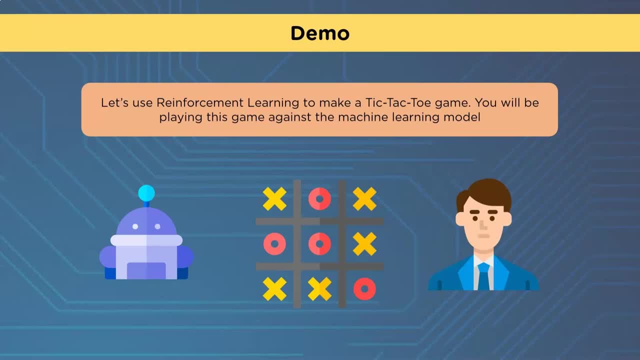 And we'll go ahead, and we're doing it in Python. So let's go ahead and go through my always- not always- I actually have a lot of Python tools. Let's go through Anaconda, which will open up a Jupyter notebook. It seems like a lot of steps, but it's worth. 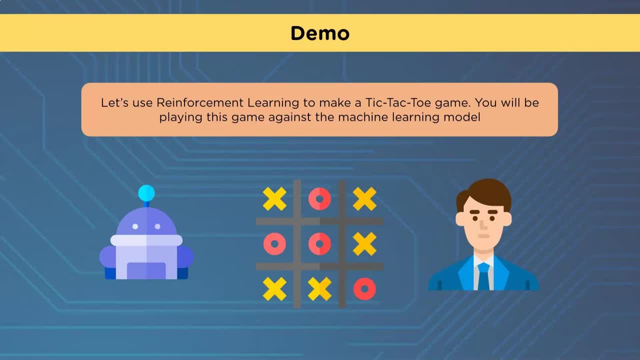 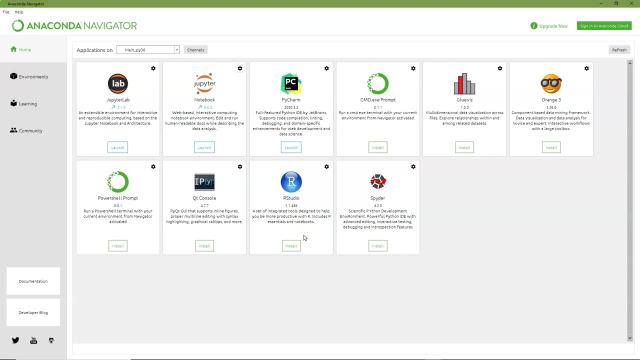 it to keep all my stuff separate And it also has a nice display when you're in the Jupyter notebook for doing Python. So here's our Anaconda navigator. I open up the notebook, which is going to take me to a web page, And I've gone in here and created a new Python tool And 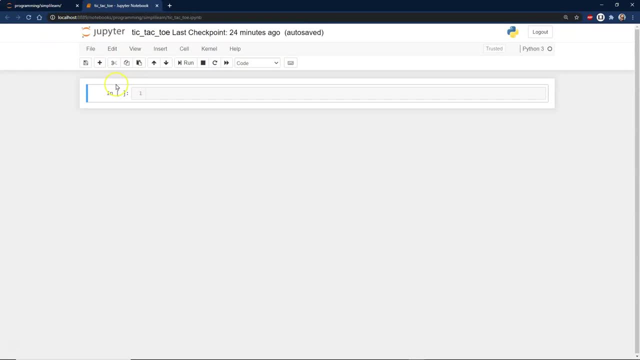 I'm going to go ahead and create a new Python tool And I'm going to go ahead and create a new Python folder- In this case, I've already done it- and enabled it to change the name to tic-tac-toe- And then, for this example, we're going to go ahead and import a couple things. We're 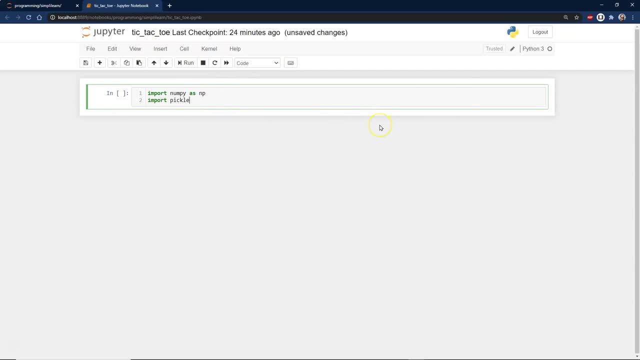 going to import numpy as np. We'll go ahead and import pickle. Numpy, of course, is our number array, And then pickle is just a nice way sometimes for storing different information, different states that we're going to go through on here, And so we're going to create a class. 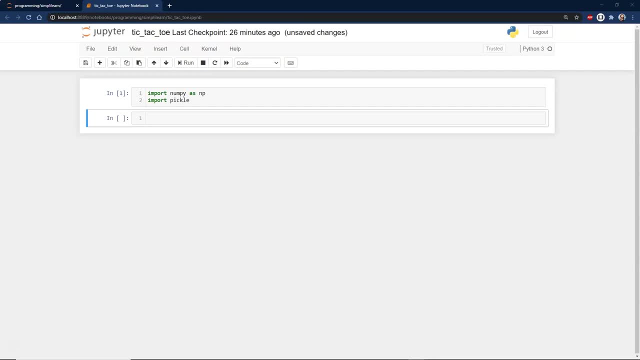 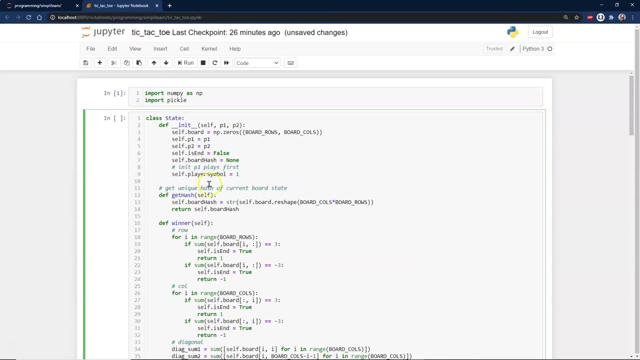 called state And we're going to start with that. And there's a lot of lines of code to this class that we're going to put in here. Don't let that scare you too much. There's not as much here. It looks like there's going to be a lot here, but there really is just a lot of setup going. 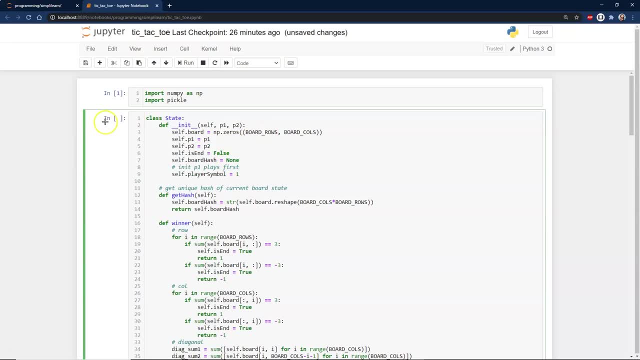 on in our class state And so we have up here. we're going to initialize it. We have our board. It's a tic-tac-toe board, So we're only dealing with nine spots on the board. We have player one. player two is end. We're going to create a board hash. We'll look at. 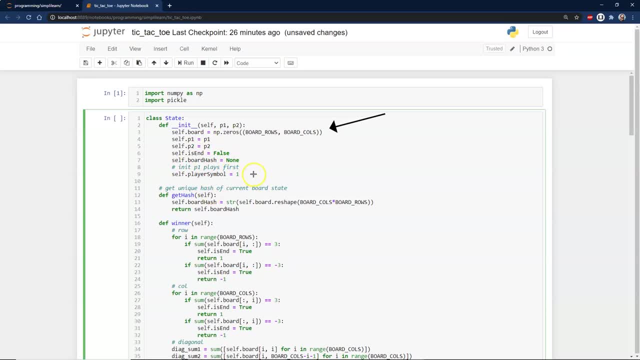 that in just a minute. We're just going to store some information in there. Symbol of player equals one, So there's a few things going on. as far as the initialization, Then something simple: We're just going to get the hash of the board. We're going to get 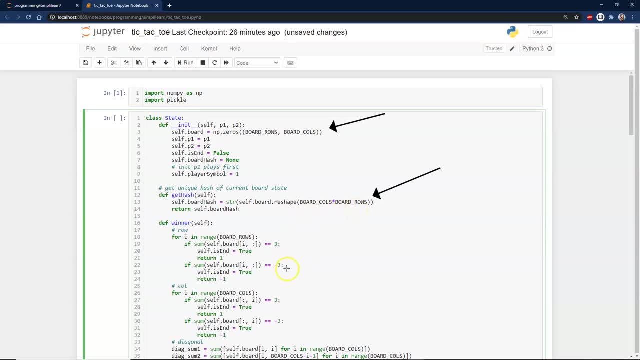 the information from the board on there, which is columns and rows. We want to know when a winner occurs. So if you get three in a row, that's what this whole section here is for. Let me go ahead and scroll up a little bit And you can get a copy of this code if 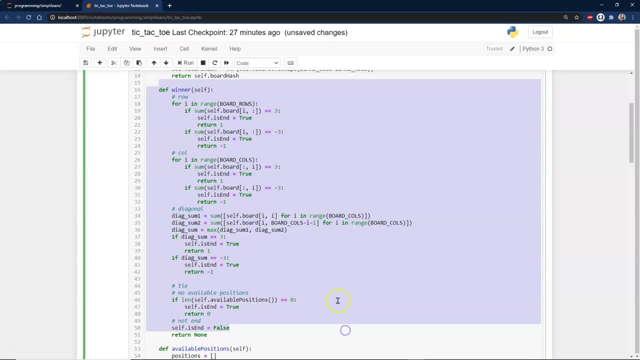 you send a note over to Simply Learn, We'll send you over this particular file and you can play with it yourself and see how it's put together. I don't want to spend a huge amount of time on this, because this is just some real general Python coding, But you can. 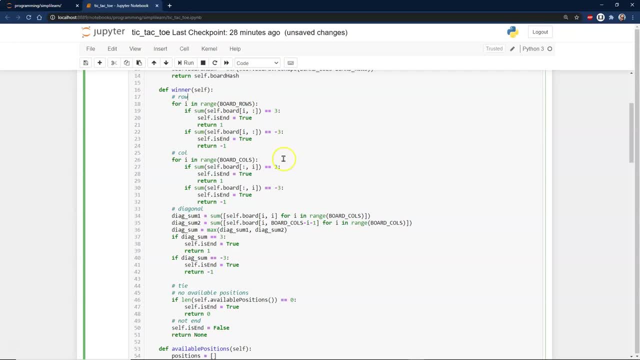 see, here we're just going through all the rows and you add them together And if it gets three in a row, same thing with columns Diagonal, so you've got to check the diagonal. That's what all this stuff does here is it just goes through the different areas Actually. 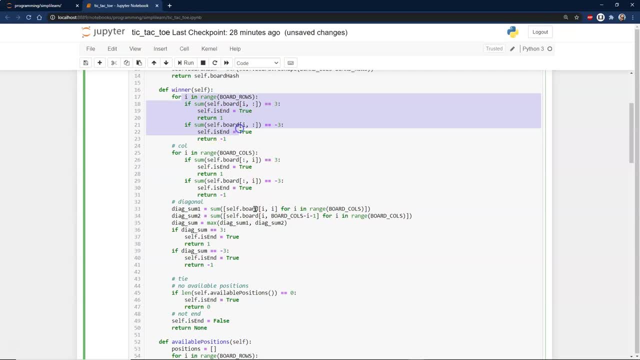 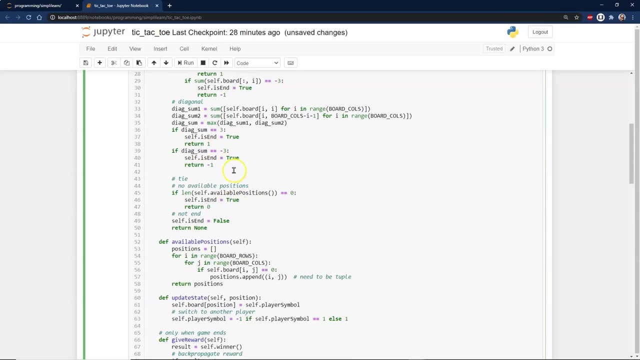 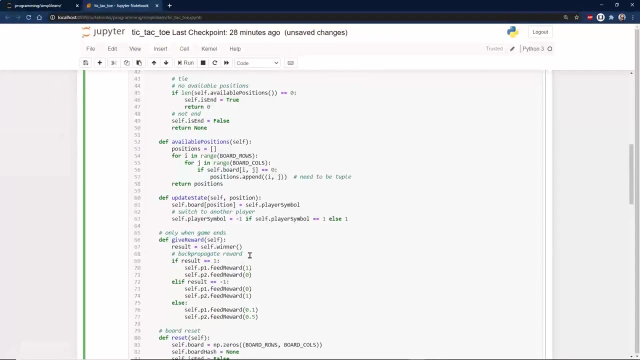 let me go ahead and put: There we go, And then it comes down here and we do our sum and it says: true Minus three just says: did somebody win or is it a tie? So you've got to add up all the numbers on there anyway, just in case they're all filled up. And next, 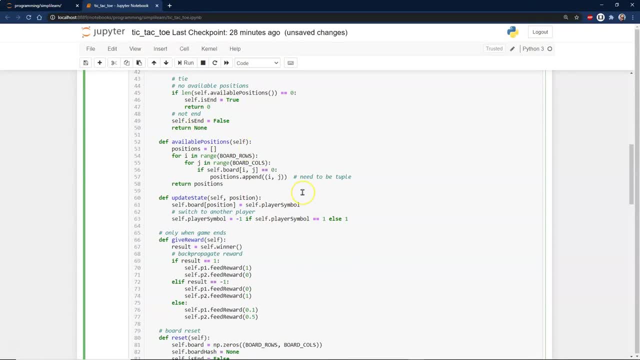 we also need to know available positions. These are ones that no one's ever used before. This way, when you try something, or the computer tries something, it's not going to give it an illegal move. That's what the available positions is doing. Then we want to update our state, And so you have your position going. 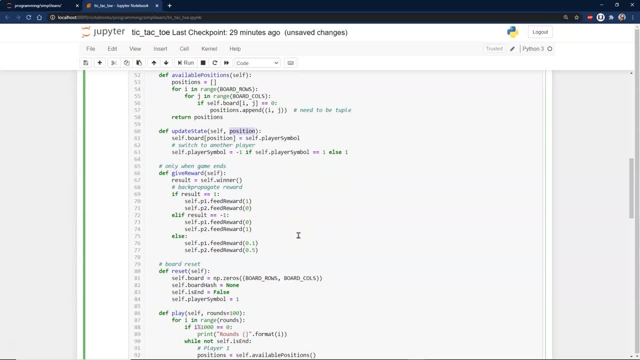 in. We're just sending in the position that you just chose And you'll see, there's a little user interface we put in there, We pick the row and column in there And again this is a lot of code. So really it's kind of a thing you'd want to go through and play with a little bit and 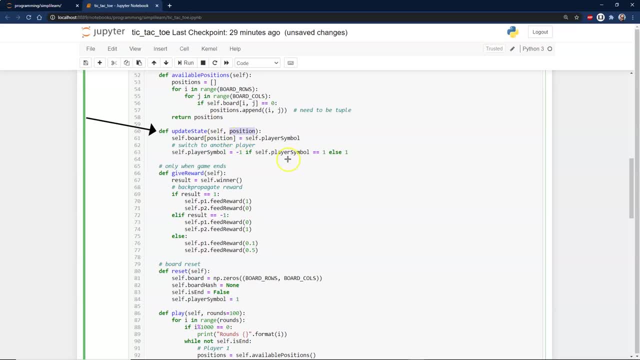 just read through it, get a copy of it- A great way to understand how this works. And here is a given reward. So we're going to give a reward. result equals self winner. This is one of the hearts of what's going on here is we have a result selfwinner. 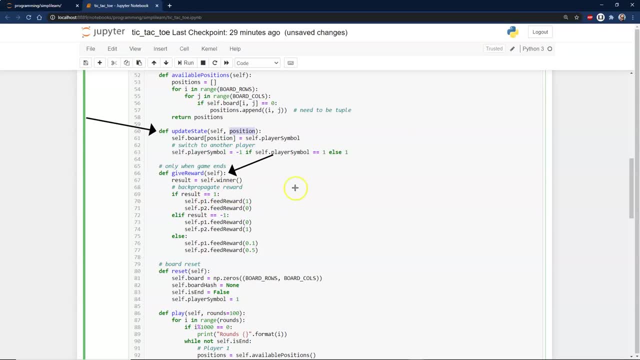 So if there's a winner, then we have a result. If the result equals one, here's our feedback. If it equals one, then it gets a zero. So it only gets a reward in this particular case if it wins. And that's important to know, because different systems of reinforced learning do. 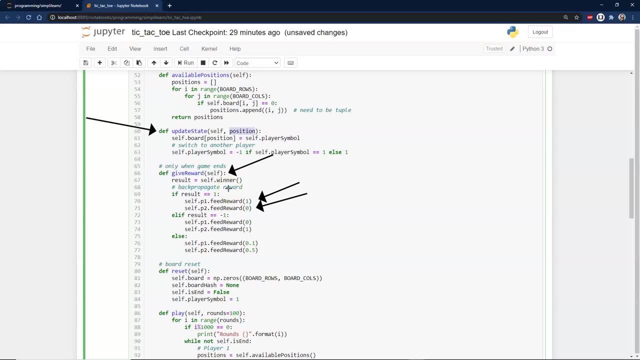 rewarding a lot differently depending on what you're trying to do. This is a very simple example with a three-by-three board. Imagine if you're playing a video game. Certainly, you only have so many actions, but your environment is huge. You have a lot going on. You have 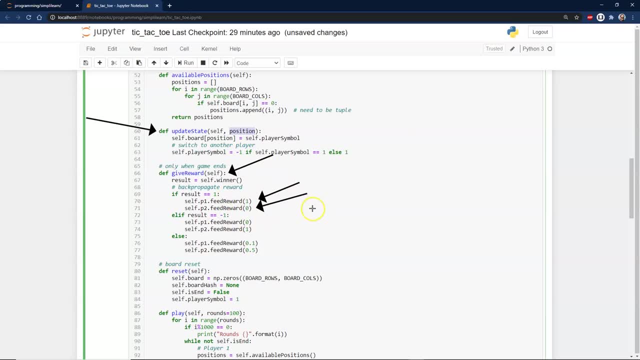 so much going on in the environment And suddenly a reward system like this is going to be just, it's going to have to change a little bit. It's going to have to have different rewards and different setup, And there's all kinds of advanced ways to do that. as far as 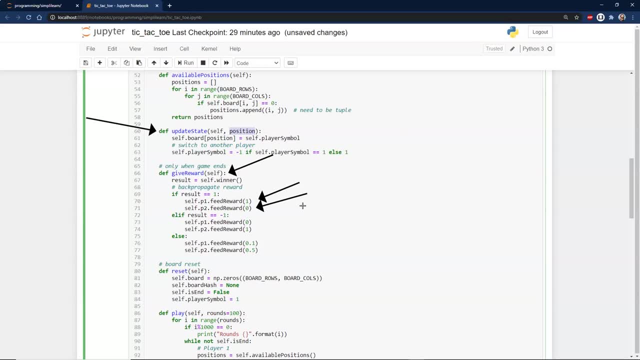 weighing, you add weights to it, And so they can add the weights up, depending on where the reward comes in. So it might be that you actually get a reward. In this case, you get the reward at the end of the game, And I'm spending just a little bit of time on this. 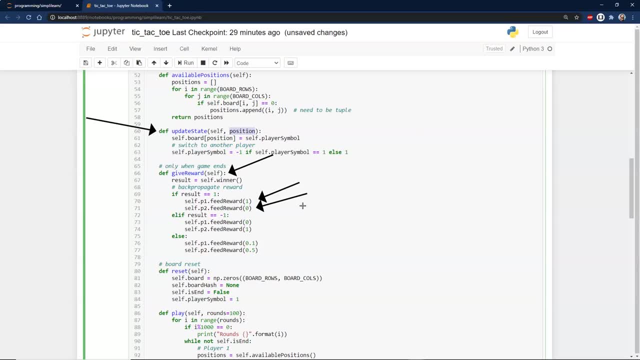 because this is an important thing to note. But there's different ways to add up those rewards. It might have like, if you take a certain path, the first reward is going to be weighed a little bit less than the last reward, because the last reward is actually winning the game or scoring or whatever it. 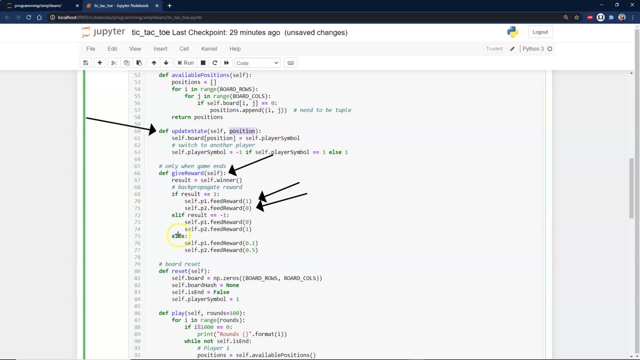 is, So this reward system gets really complicated in some of the more advanced setups. In this case, though, you can see right here that they give a .1 and a .5 reward just for getting a pick in the right value and something that's actually valid, instead of picking an invalid. 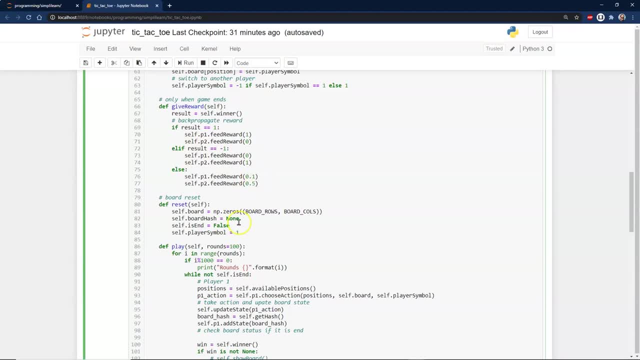 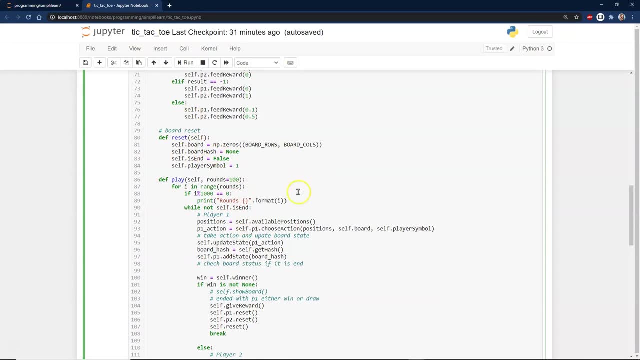 value. So rewards again. that's like key. It's huge. How do you feed the rewards back in? Then we have a board reset. That's pretty straightforward. It just goes back and resets the board at the beginning because it's going to try out all these different things while it's learning. 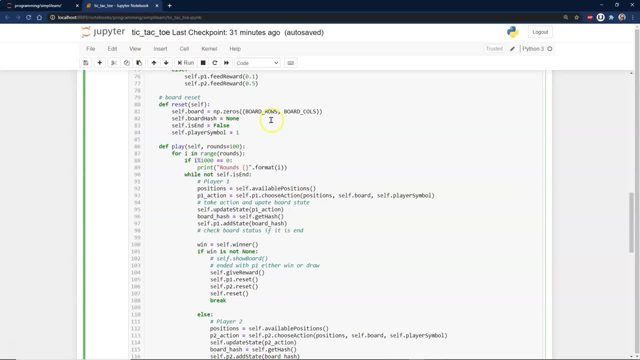 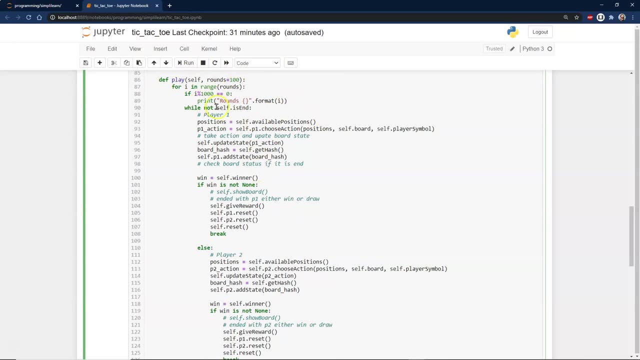 It's going to do it by trial and error, So you have to keep resetting it. And then, of course, there's the play. We want to go ahead and play Rounds equals 100.. Depends on what you want to do on here. 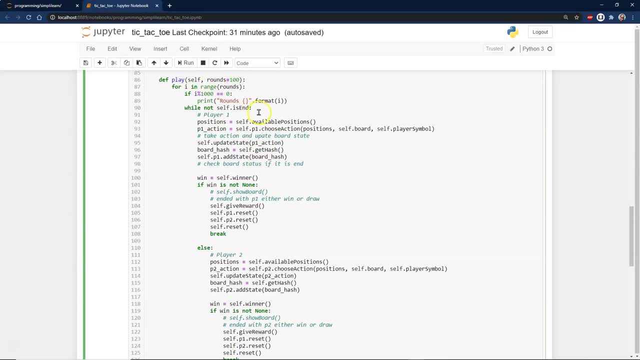 You can set this different. You can obviously set that to higher level, But this is just going to go through and you'll see in here that we have player one and player two. This is the computer playing itself, One of the more powerful ways to learn to play a game. 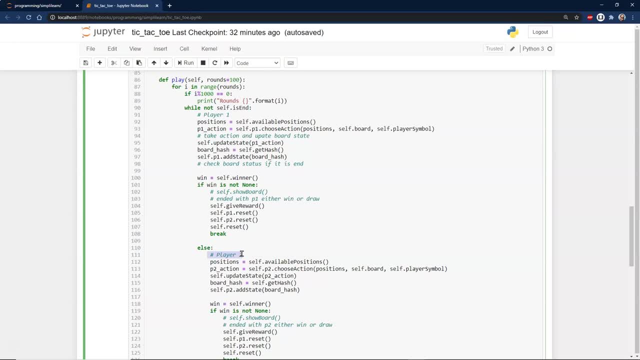 or even learn something. that isn't a game is to have two of these models that are basically trying to beat each other, And so they always. they keep finding, exploring new things. They're all the same. This one works for this one. So this one tries new things, It beats this. 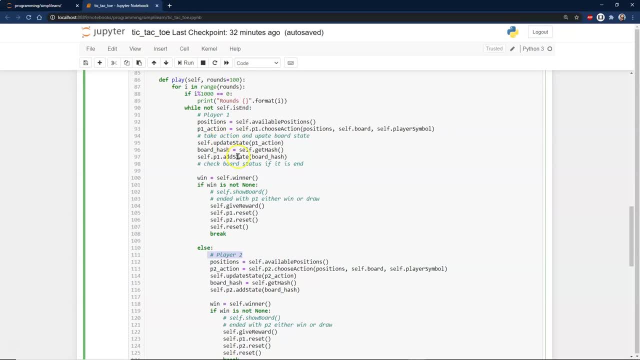 We've seen this in chess. I think was a big one where they had the two players in chess with reinforcement learning. It was one of the ways they trained one of the top computer chess playing algorithms. So this is just what this is: It's going to choose an action. 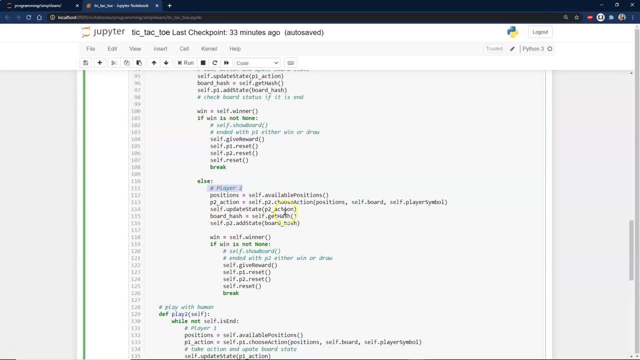 It's going to try something And the more it tries stuff, the more we're going to record the hash. We actually have a board hash where they can self get the hash set up on here. It stores all the information And then once you get to a win- one of them wins, It gets. 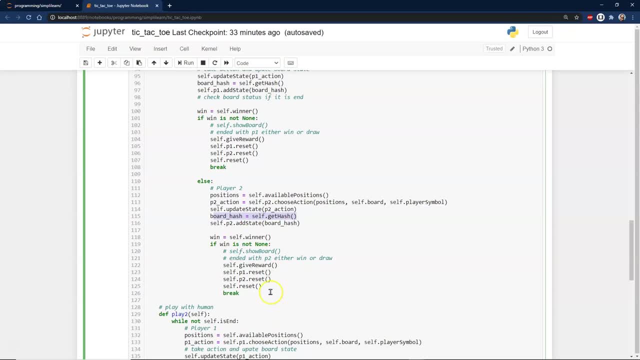 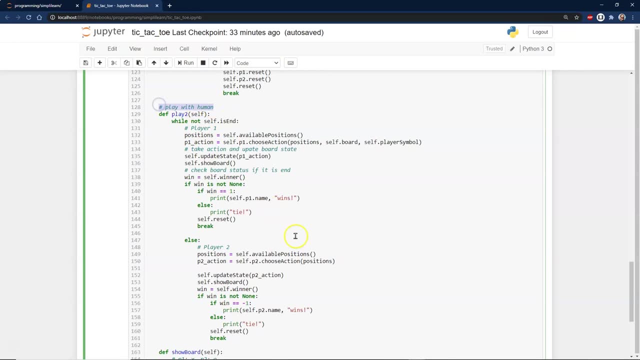 the reward. Then we go back and reset and try again And then kind of the fun part we actually get down here is we're going to play with a human, So we'll get a chance to come in here and see what that looks like when you put your own information in. And then 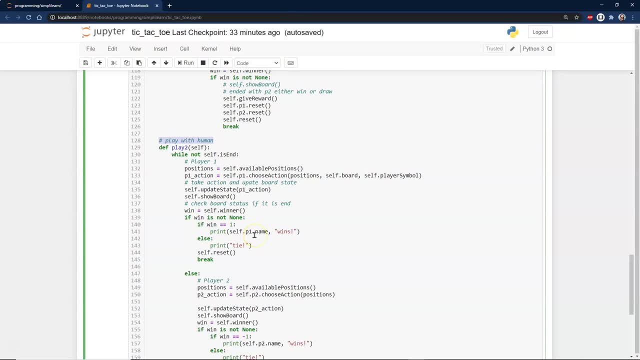 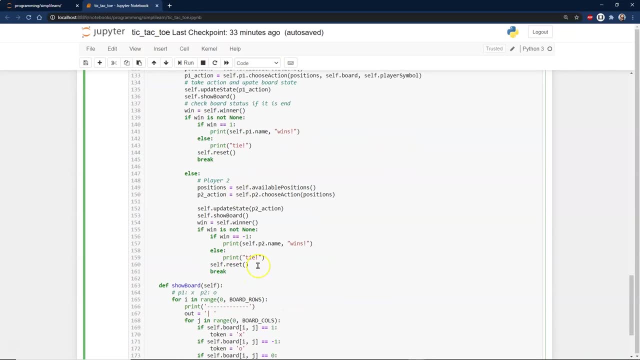 it just comes in here and does the same thing it did above. It gives it a reward for its things or sees if it wins or ties, Looks at available things, All that kind of fun stuff. And then, finally, we want to show the board. So it's going to. 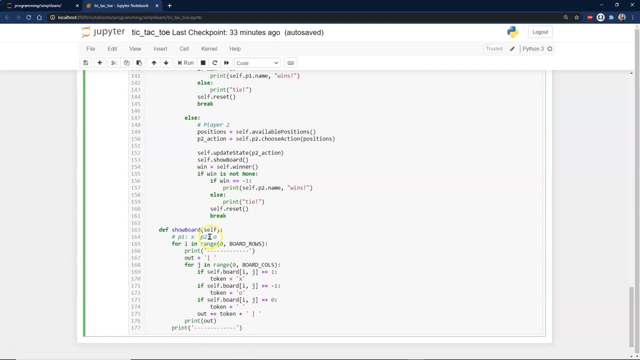 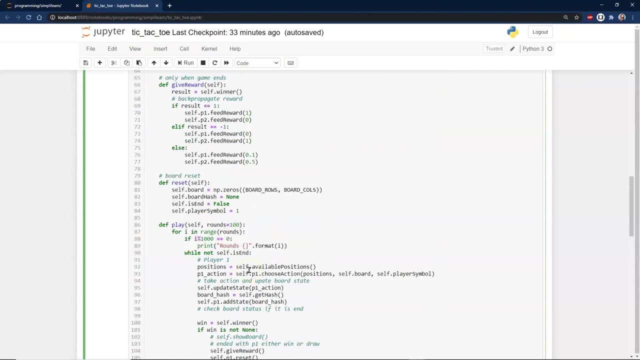 print the board out each time, Really, as an integration. it's not that exciting. What's exciting in here is one looking at this reward system. Whoops, play one more up. The reward system is really the heart of this. How do you reward the different set up And the other? 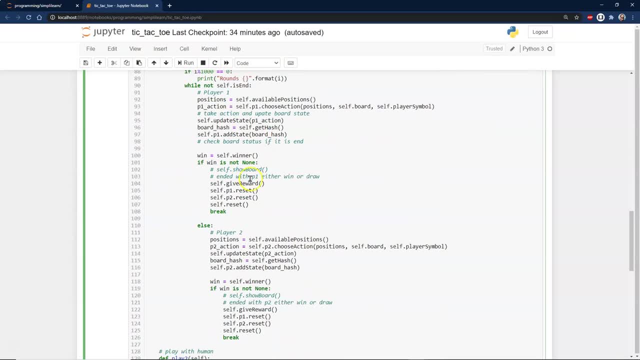 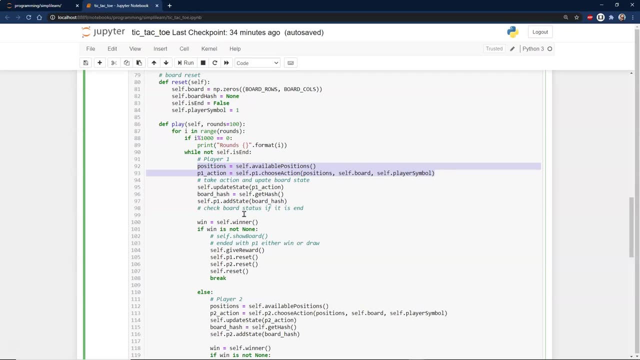 one is when it's playing. it's got to take an action, And so what it chooses for its actions is also the heart of reinforcement learning. How do we choose that action? And those are really key to right now, where reinforcement learning is in today's technology. 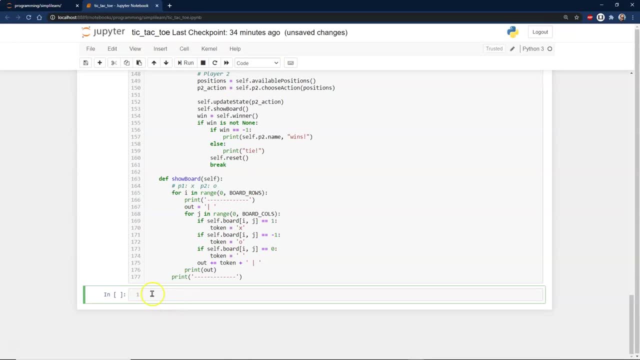 Figuring this out. How do we reward it and how do we guess the next best action? So we have our environment. You can see the environment iswe're going to be here with the state which is kind of like what's going on. 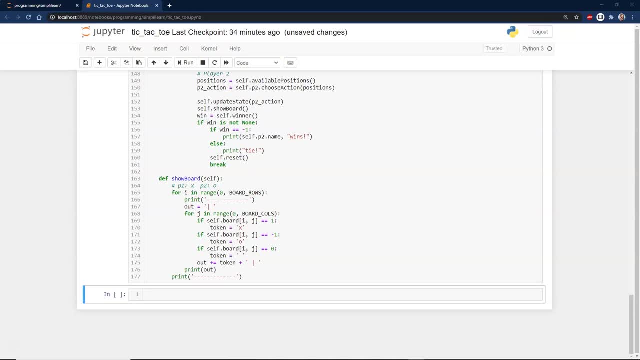 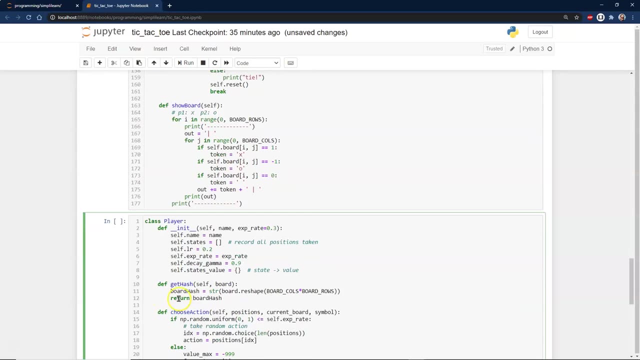 We're going to return the state, depending on what happens, And we want to go ahead and create our agent, In this case, our player. So each one is: let me go ahead and grab that, And so we look at a class player. 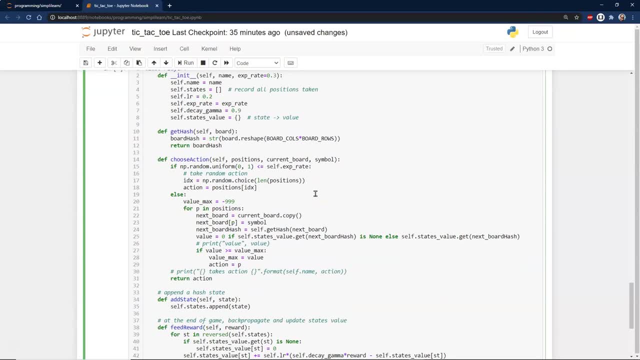 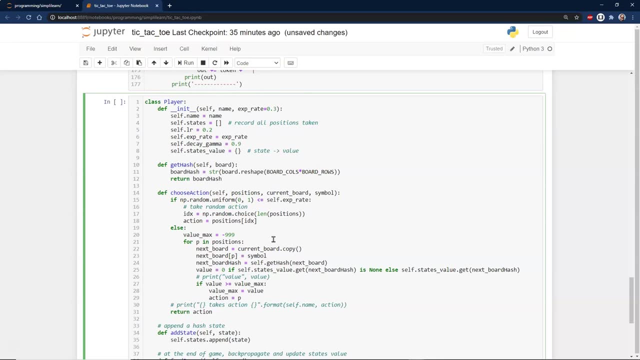 This is where a lot of the magic is really going on is how is this player figuring out how to maneuver around the board, And then the board, of course, returns a state that it can look at and reward. So we want to take a look at this. 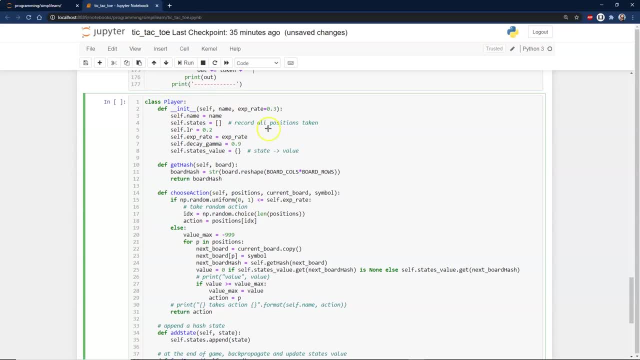 We have name self-state. this is class player. And when you say class player, we're not talking about a human player, We're talking about just the computer players, And this is kind of interesting. So, remember, I told you, depending on what you're doing, 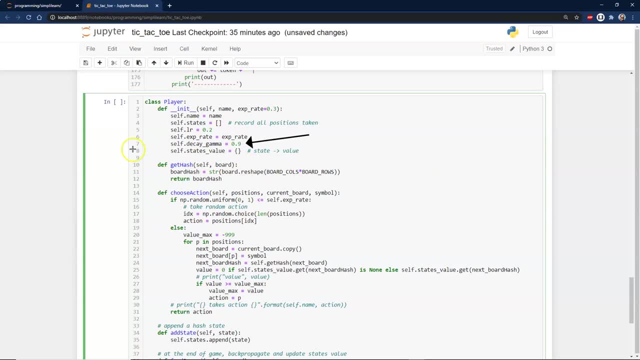 there's going to be a decay gamma explore rate. These are. what I'm talking about is how do we train it? As you try different moves, it gets to the end And the first move. it is important, but it's not as important as the last one. 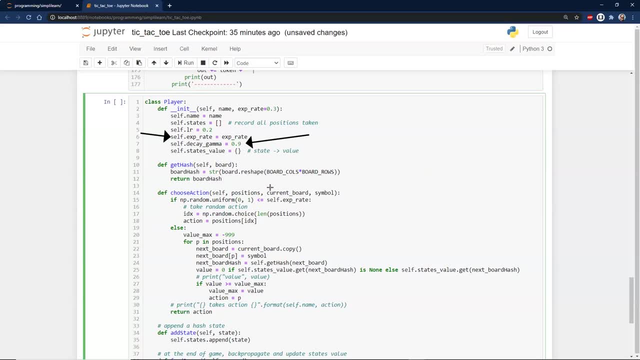 And so you could say that the last one has the heaviest weight. And then, as you get there, the first one- let's say the first move- gives you a five reward, The second gives you a two reward, And the third one gives you a 10 reward, because that's the final ending. 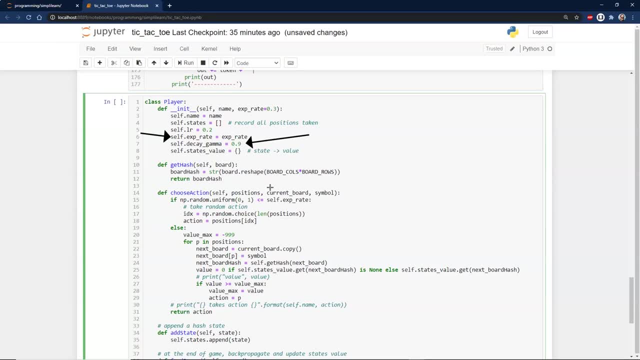 You got it. The 10 is going to count more than the first step, And here's our: we're going to get the board information coming in and then choose an action. This was the second part that I was talking about. that was so important. 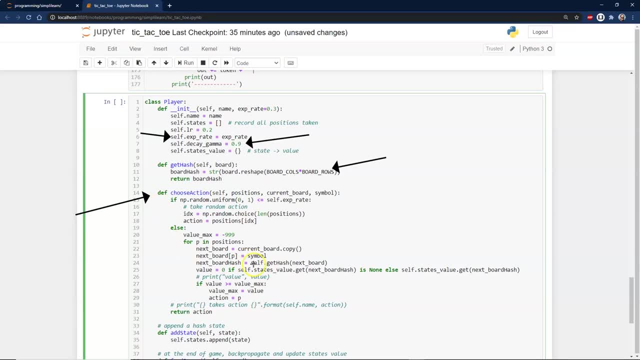 So once you have your training going on, we have to do a little randomness and you can see, right here is our NP random uniform. So it's picking out a random number, take a random action. This is going to just pick which row and which column it is. 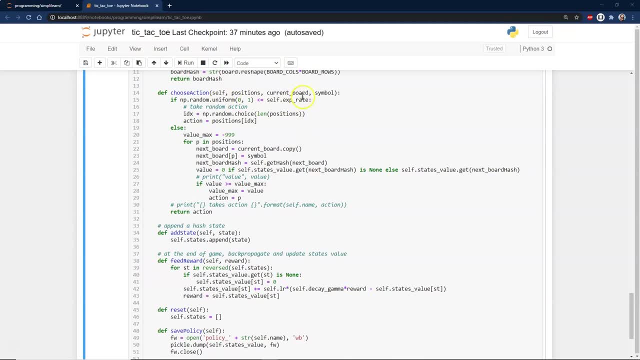 And so choosing the action, this one. you can see we're just doing random states choice, length of positions, action position. And then it skips in there and takes a look at the board For P and positions. it's actually storing the different boards each time you go through. 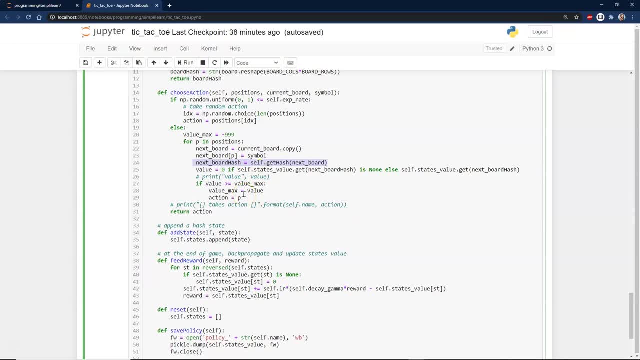 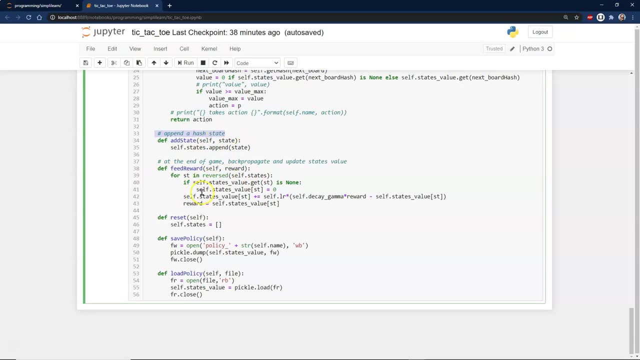 So it has a record of what it did, so it can properly weigh the values. And this simply just appends a hash state. What's the last state? Append it to the, to our states on here. Here's our feedback: rewards. The reward comes in and it's going to take a look at this and say: is it none? 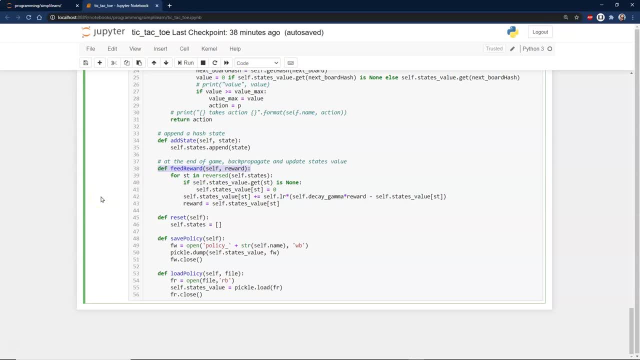 What is the reward? And here is that formula, Remember I was telling you about up here. It was important because it has decay gamma times. the reward: This is where, as it goes through each step, and this is really important, This is- this is kind of the heart of this, of what I was talking about earlier. 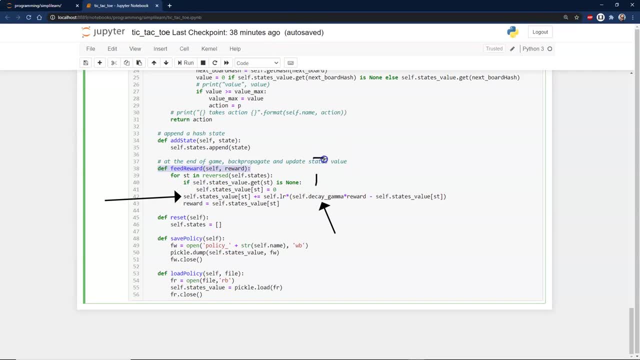 You have step one, and this might have a reward of two. You have step two. I probably should have done ABC. This has a step three, step four and so on, So you get to step in and this might have a reward of 10.. 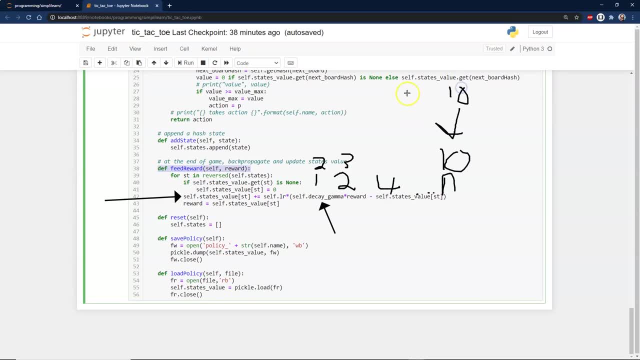 So reward of 10, we're going to add that, but we're not adding. let's say this one right here. Let's say this reward here before 10 was, let's say it's also 10.. That just makes the math easy. 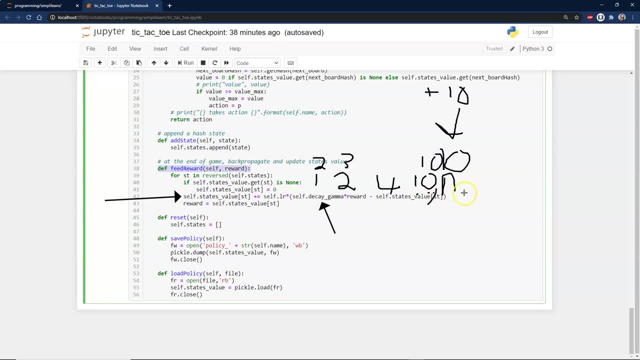 So we had 10 and 10.. We had 10.. This is 10 and 10N, whatever it is, But it's time, It's 0.9.. So instead of putting a full 10 here, we only do nine. 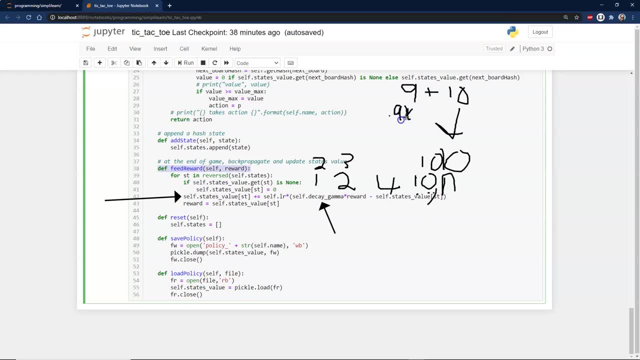 That's 0.9 times 10.. And so this formula, as far as the decay times the reward minus the cell state value, it basically adds in, it says: here's one or here's two. I'm sorry, I should have done this ABC. 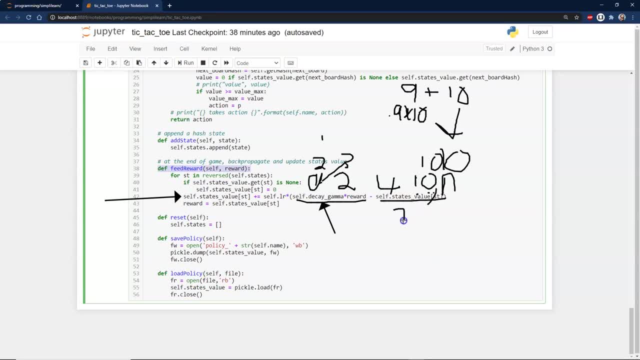 It would have been easier. So the first move goes in here And it puts two in here. Then we have our self set up on here. You can see how this gets pretty complicated in the math. But this is really the key is: how do we train our states? 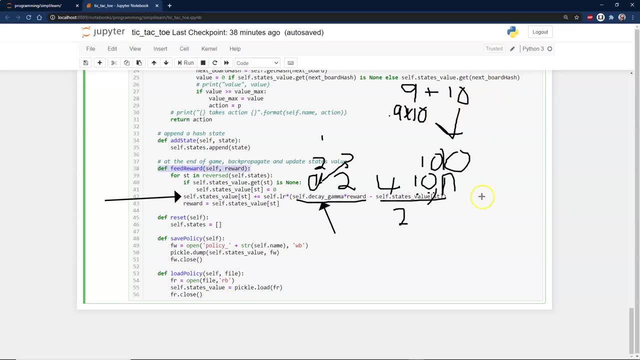 And we want the final state, the win, to get the most points. If you win, you get most points And the first step gets the least amount of points. So you're really training this almost in reverse. You're training it from the last place where you have like a point. 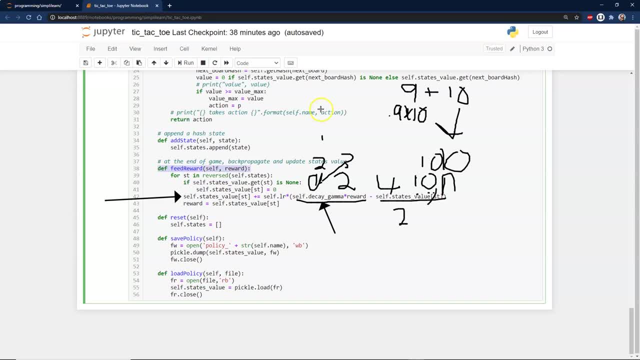 You're training it from the last place where you have like a point. What happens when you fry? You change it. What happens when you fry that point? It gets greener. So it's hard because they can't see that point. 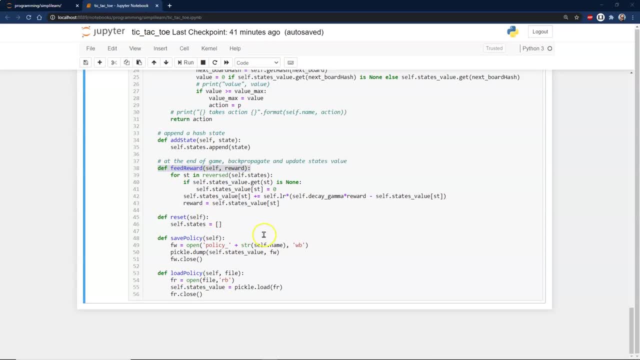 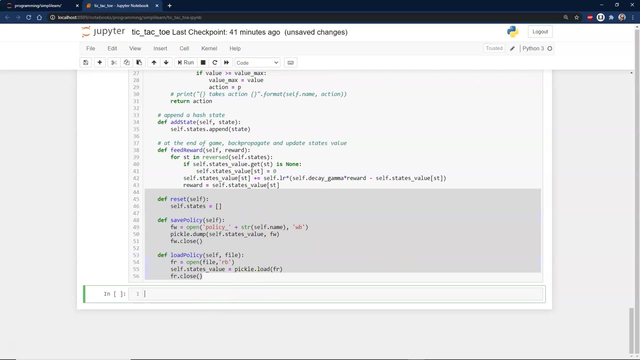 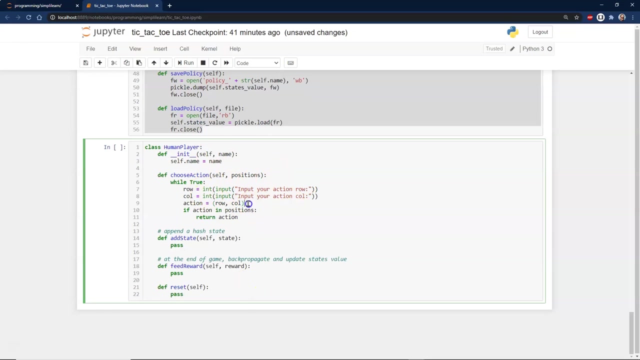 So I change it from green. So it get's sundown and it gets darker. So after every single throw, What happens? go ahead and create a human player, And the human player is going to be a little different in that you choose an action row and column. here's your action. If action is if action. 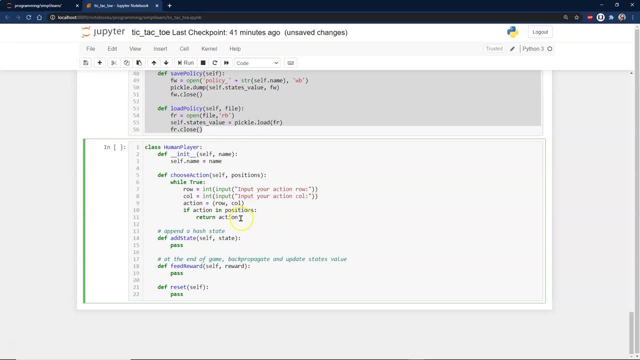 in positions- meaning positions that are available- you return the action. If not, it just keeps asking you until you get an action that actually works, And then we're going to go ahead and append to the hash state, which we don't need to worry about because it returns the 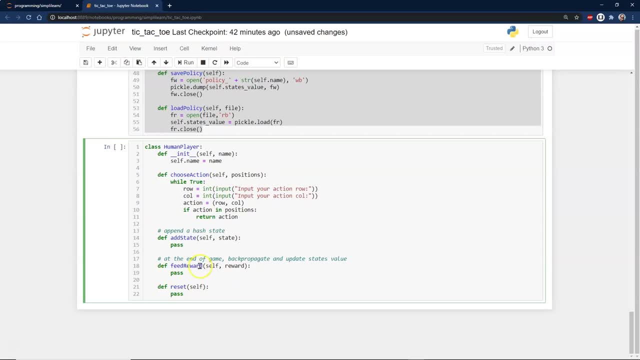 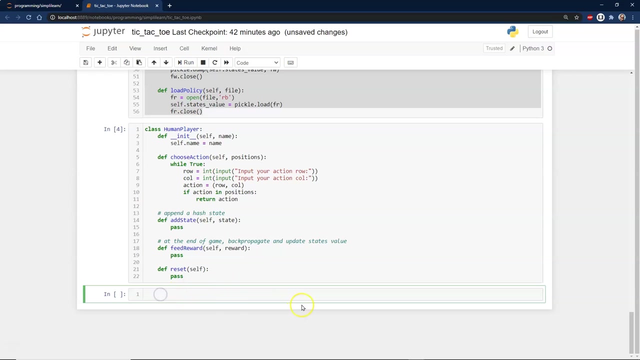 action up here and feed forward Again this is because it's a human at the end of the game- bat, propagate and update state values. This part isn't being done because it's not programming the model. The model is getting its own rewards, So we've gone ahead and loaded. 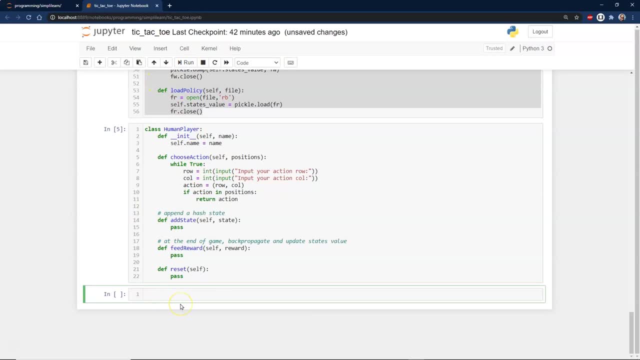 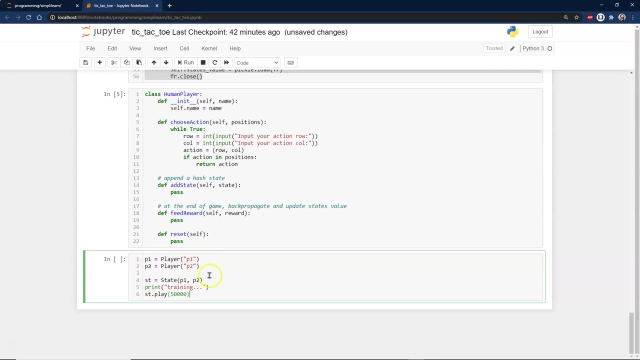 this in here. So here's all our pieces, And the first thing we want to do is set up P1 player 1, P2 player 2, and then we're going to send our players to our state. So now it has P1, P2, and it's going to play, and it's going to play 50,000 rounds Now. 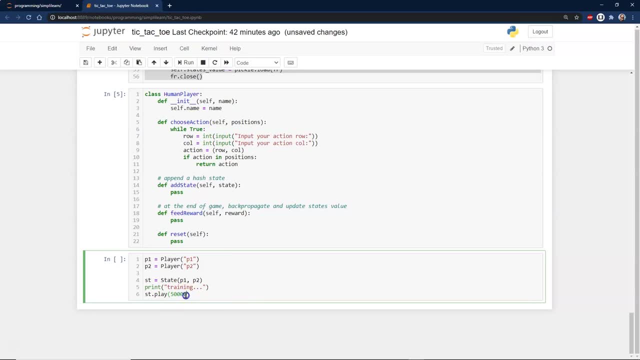 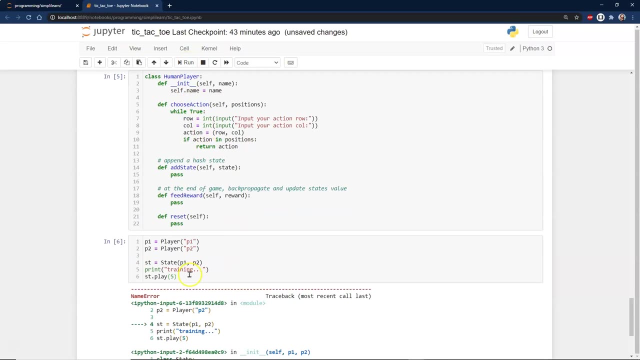 we can probably do a lot less than this, and it's not going to get the full results. In fact, you know what? let's go ahead and just do 5, just to play with it, because I want to show you something here. Oops, somewhere in there I forgot to load something. 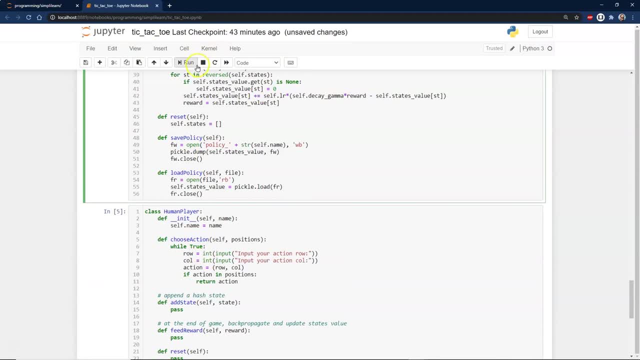 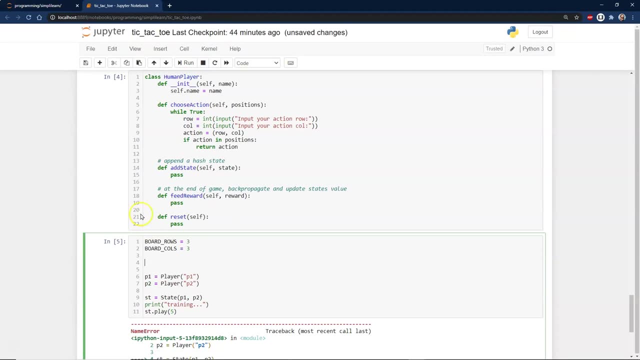 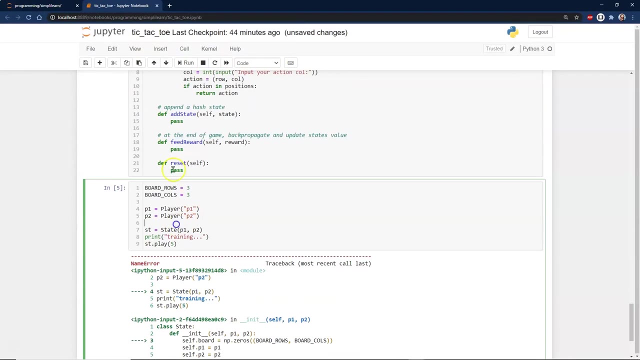 There we go. I forgot to run this. Oops, forgot a reference there for the board rows and columns three by three. There's actually in the state it references that We can just tack it on on the end. It was supposed to be at the beginning, So now I've only set. 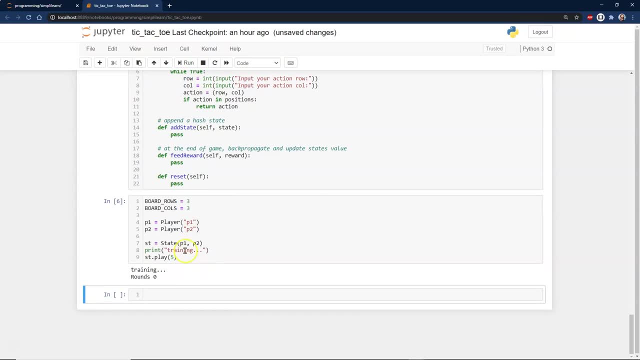 this up with. let's see where are we going here. I've only set this up to train the player five times, And the reason I did that is we're going to come in and actually play it and then I'm going to change that and we can see how it differs on there There. 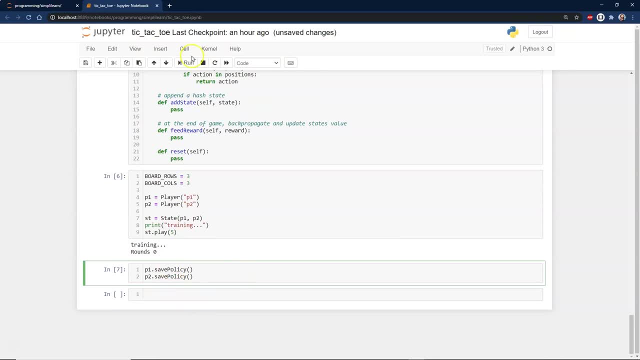 we go. It didn't even make it through a run and we're going to go ahead and save the policy. So now we have our player 1 and our player 2 policy. The way we set it up, it has two separate policies loaded up in there, And then we're going to come in here and we're 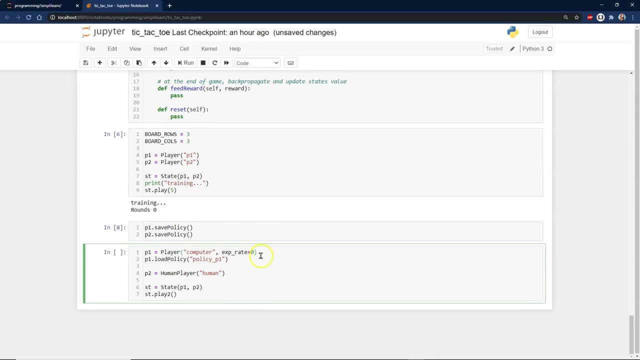 going to do. player 1 is going to be the computer experience rate, zero load policy, one human, player, human, and we're going to go ahead and play this Now. remember, I only went through it. just one round of training, in fact, minimal training, And so it puts an X there and I'm 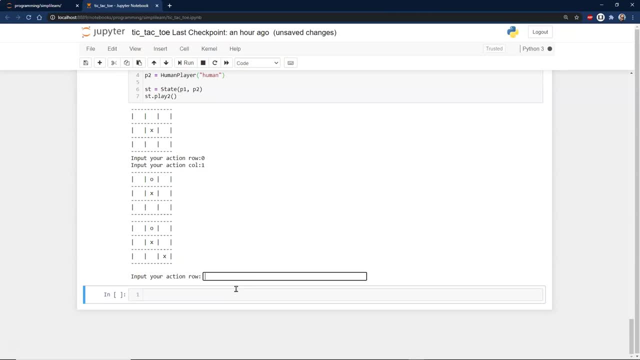 going to go ahead and do row zero, column one, And you can see this is very basic on here, And so I put in my zero and then I'm going to go zero, block it zero And then zero, And you can see, right here it let me win. Just like that I was able to win. 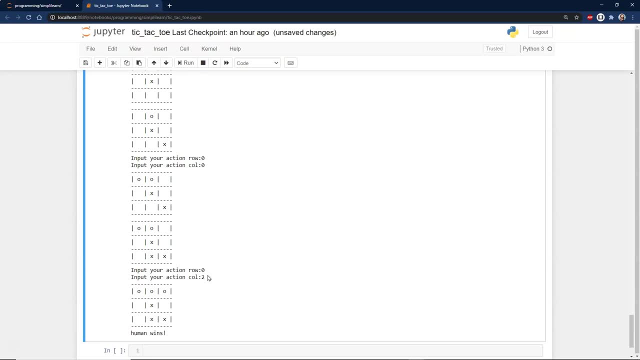 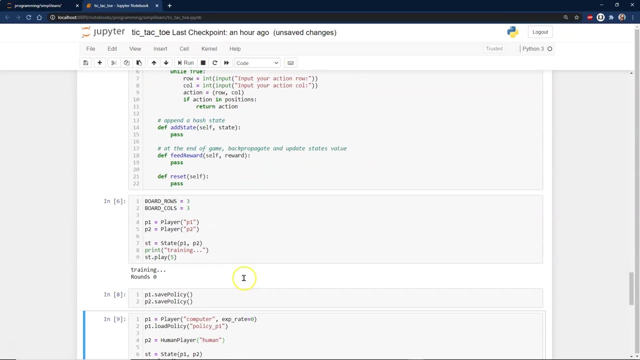 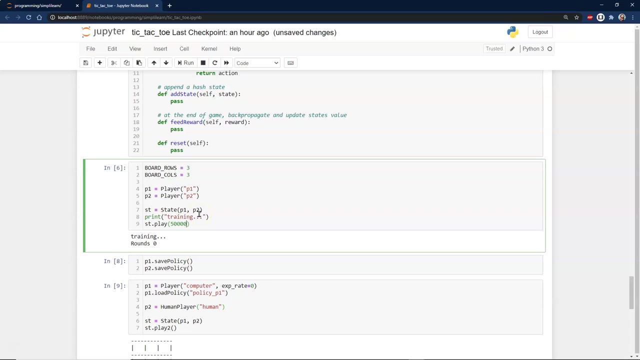 Zero two and whoo human wins. So I only trained it five times. We're going to run this again, and this time, instead of five let's do 5,000, or 50,000.. I think that's. 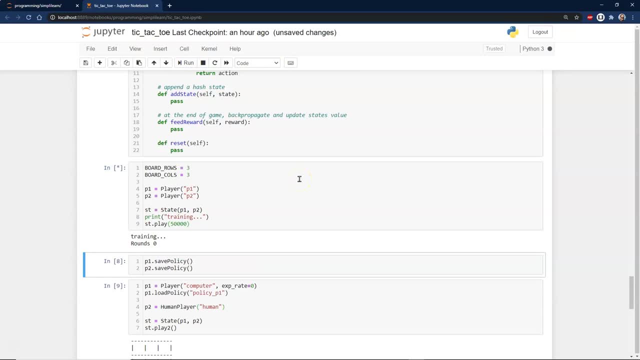 what the guys in the back had, And this takes a while to train it. This is where really reinforcement learning really falls apart. Look how simple this game is. We're talking about a three-by-three set of columns, And so for me to train it on this, I could do. 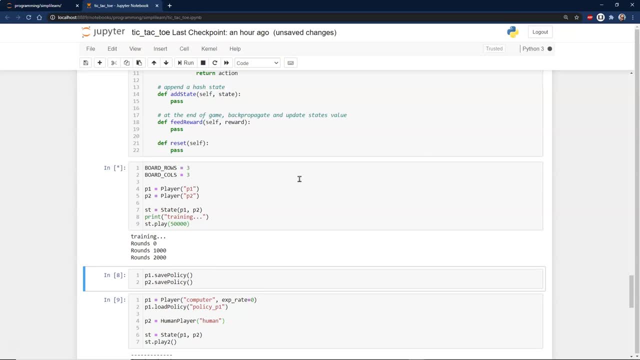 a cue table, which would go much quicker. You could build a quick cue table with almost all the different options on there and you would probably get the same result much quicker. We're just using this as an example. So when we look at 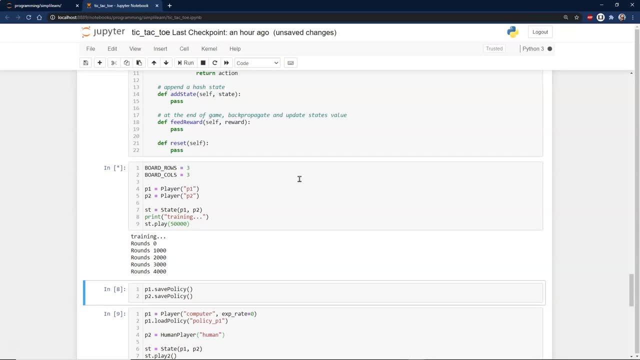 reinforcement learning. you need to be very careful what you apply it to. It sounds like a good deal until you do a large neural network where you set the neural network to a learning increment of one, So every time it goes through it learns, And then you do your actions. You 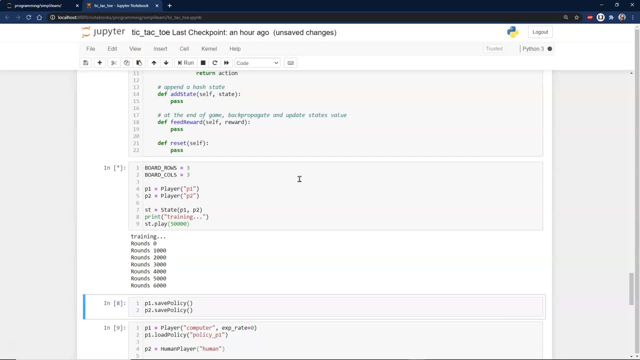 pick from the learning setup and you actually try actions on the learning setup until you get what you think is going to be the best action. So you actually feed what you think is right back through the neural network. There's a whole layer there which is really fun to play with And then it has an output. Well, think of all those. 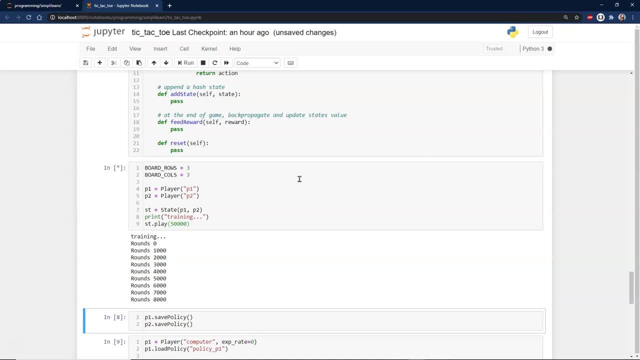 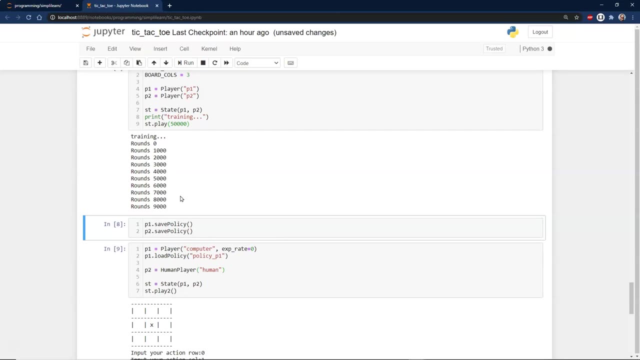 processes. I mean that is just a huge amount of work it's going to do. Let's go ahead and skip ahead here. Give it a moment. It's going to take a minute or two to go ahead and run Now to train it. we went ahead and let it run and it took a while. 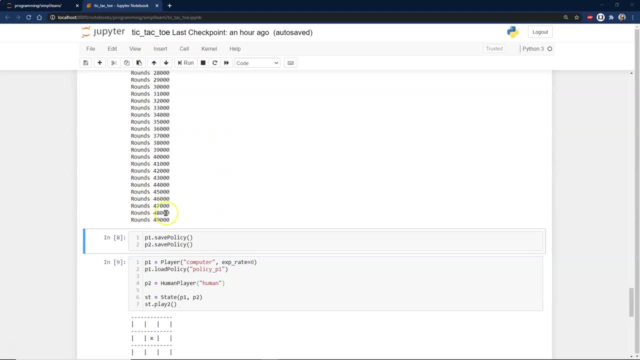 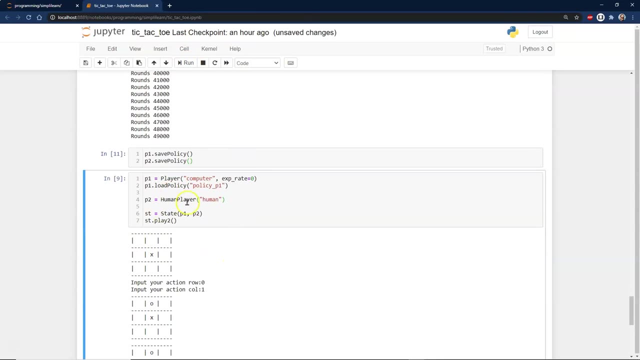 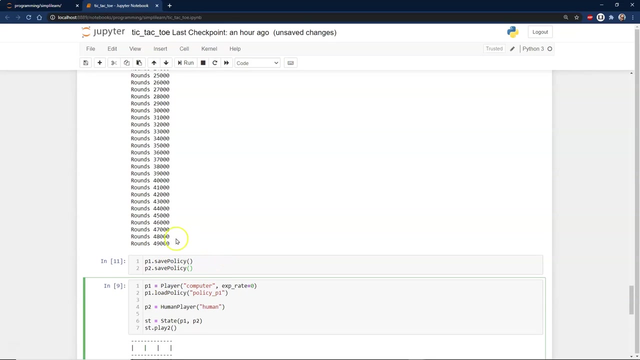 This took. I got a pretty powerful processor and it took about five minutes plus to run And it started running And we're running a little bit longer than it was supposed to run. Let's just repeating myself so that we can get a real 간단 way of thinking about how. 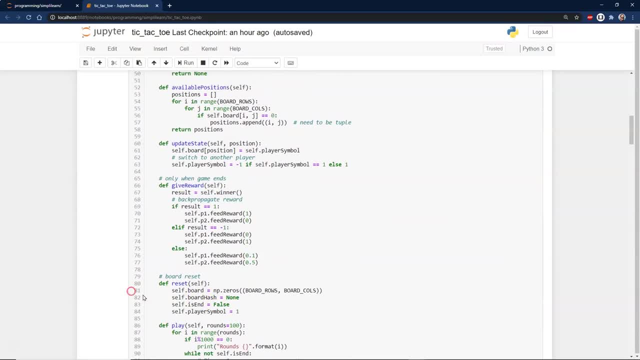 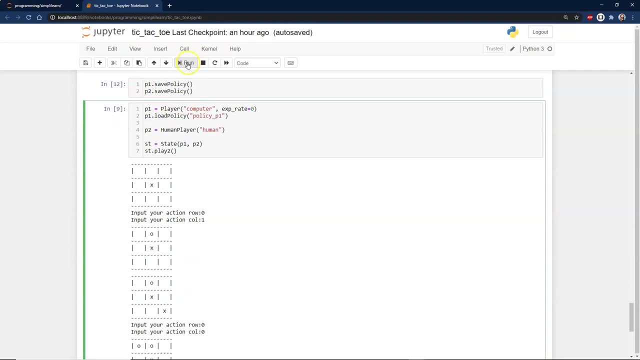 to run it And we'll go ahead and run our player setup on here. Oops, I brought in the last Whoops, I brought in the last round, So give me just a moment to redo the policy. save There we go. I forgot to save the policy back in there And then go ahead and run our player again. So we've saved the policy. Then we want to go ahead and load the policy for p1 as a computer. 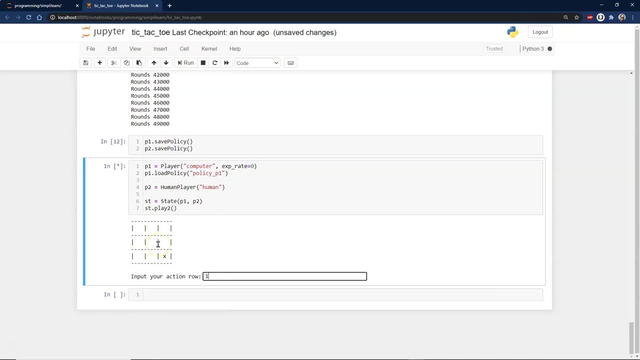 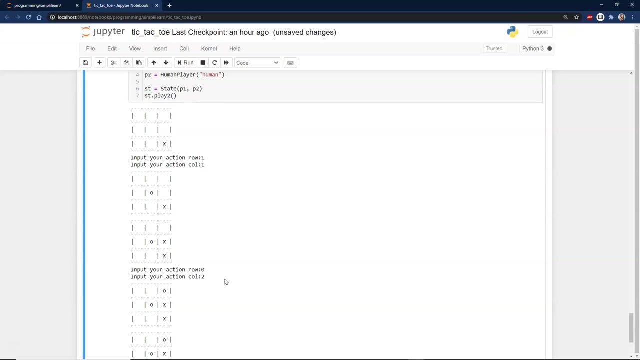 right corner. I'm gonna go ahead and go 11, which is the center, and it's gone right up the top, and if you ever played tic-tac-toe you know the computer has me, but we'll go ahead and play it out. row zero, column two: there it is, and then 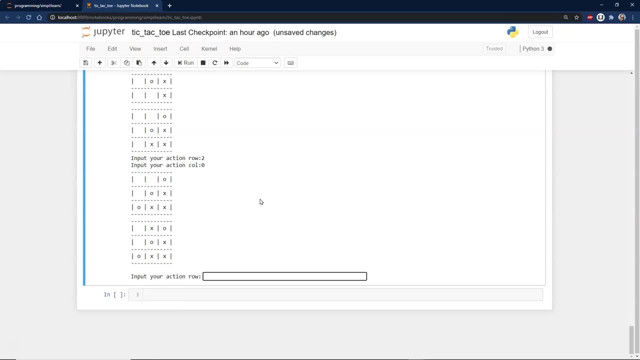 it's gone here, and so I'm gonna go ahead and go row zero one, two, no, zero one. there we go and column zero. that's where I want it. oh, and it says: I okay, you, your action. there we go, boom. so you can see, here we've got a. didn't catch the win on.